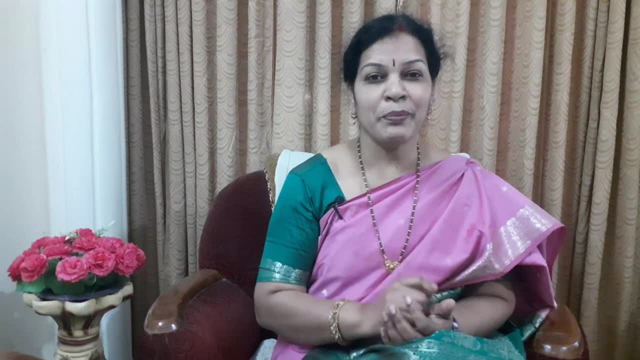 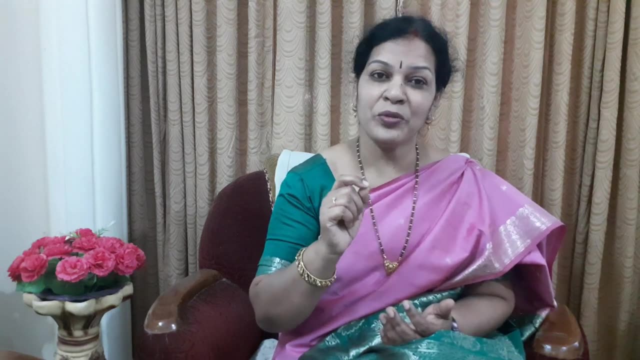 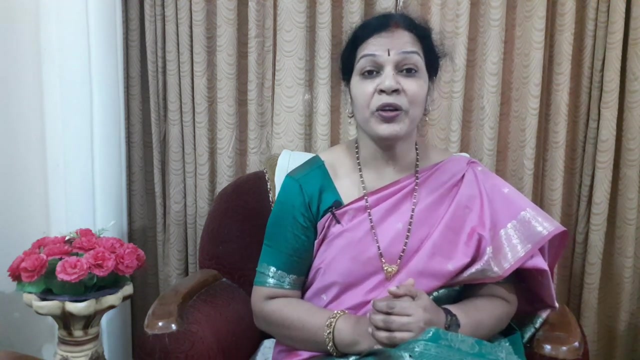 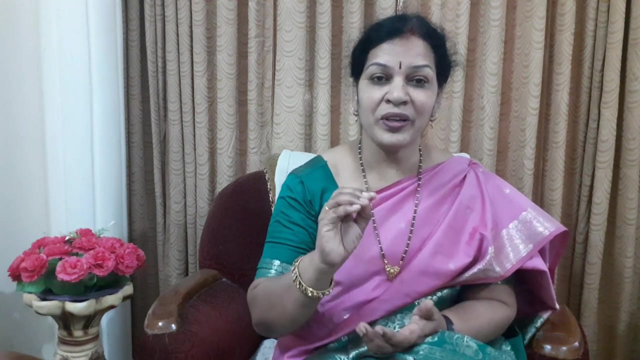 You know that teaching is one of the best profession, Respectable and remarkable, and also one of the best profession. So when you enter into the teaching field, what should be your attitude, What you have to do? This guidance nobody will give you. There is no profession, there is no book is available, But I want to guide you a few things. to all the young faculty: 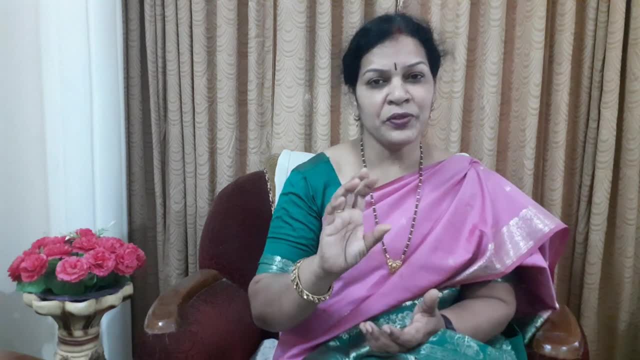 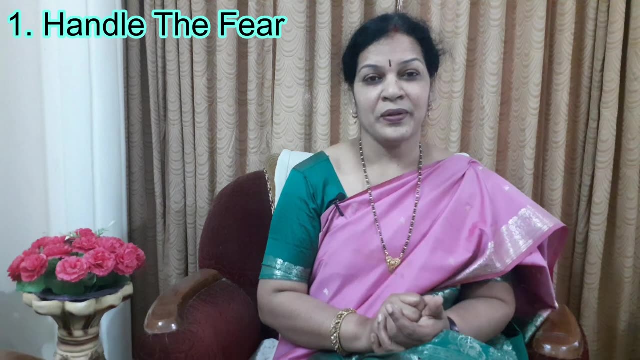 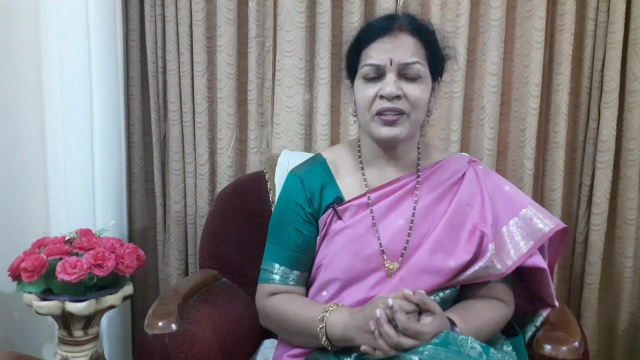 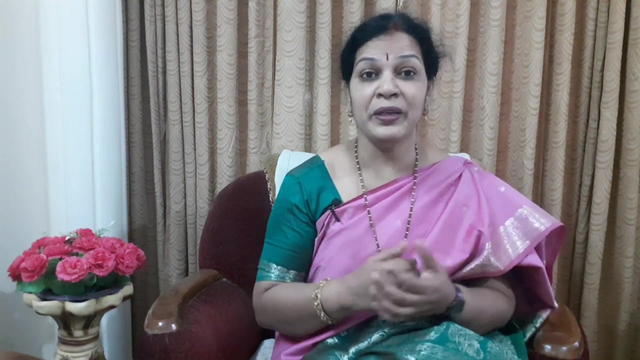 The first thing is that once, if you enter into the teaching field like, you will have a fear. Handle the fear first. When you see the students, you will have a fear. But why do you have fear? Why to have fear? They are just students. You have better knowledge, you have good knowledge, you have good qualification, you have cleared many exams. Do you accept it In front of you, students are nothing. 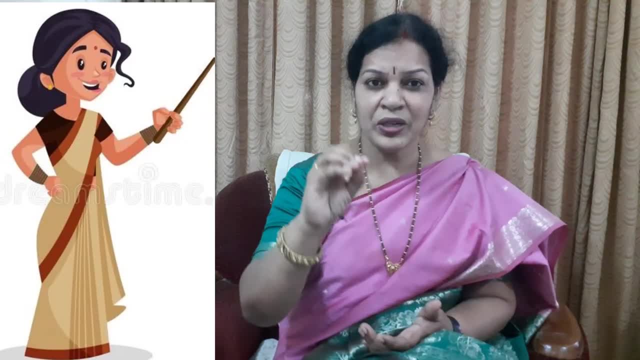 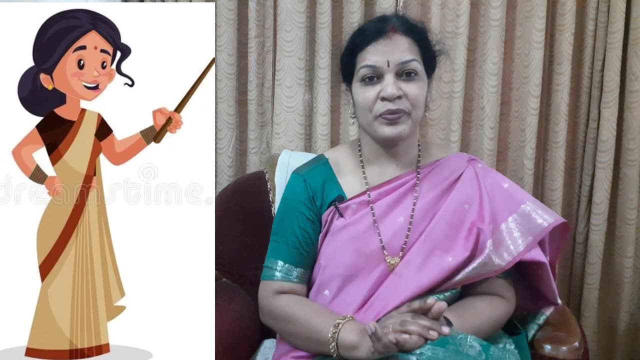 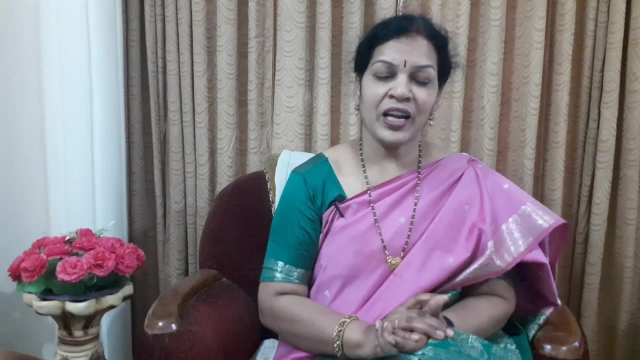 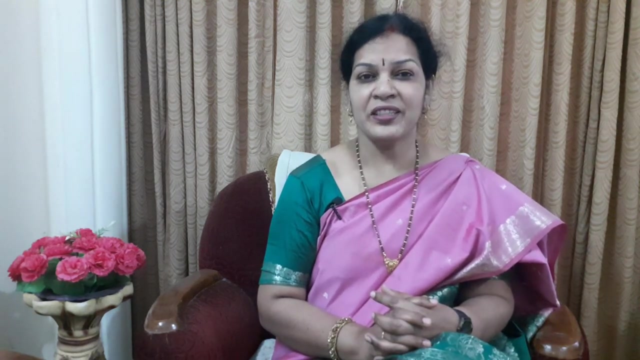 I am telling you They don't know anything. You have to train them. The moment when you feel that they don't know anything, you will not have any fear. And for teaching also, you need to have some practice. Start in front of mirror- or- nowadays technology is there- Record your lectures by yourself and see how you are teaching. how is your body language, how is your communication skills, how you are explaining the concept. 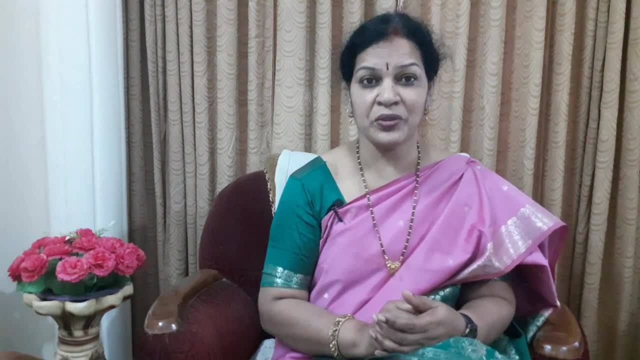 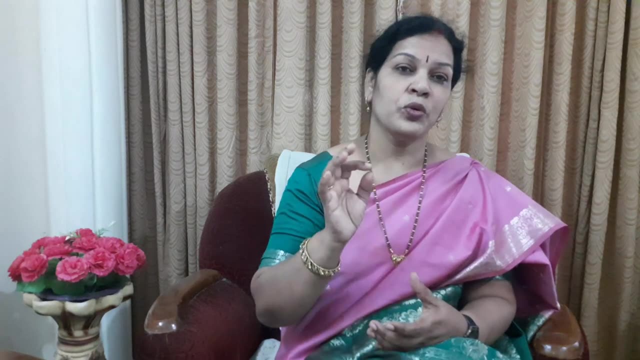 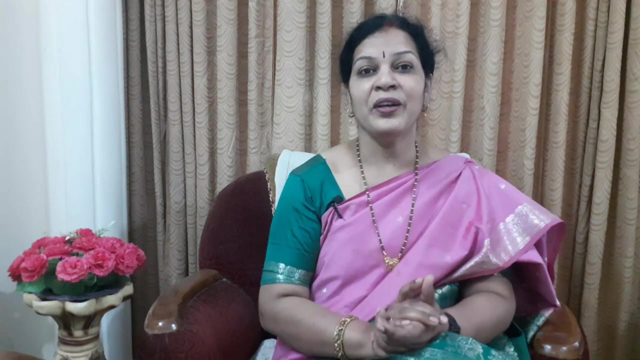 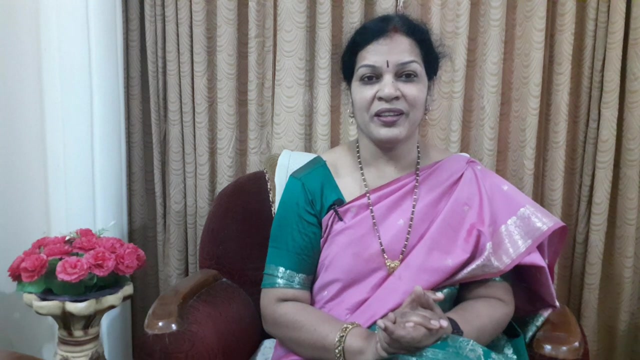 Is it understandable to a common student, average student or below average student, Like you can ask yourself some questions and you can practice it at yourself only. So never have a fear. And the moment when you enter into the class also, please cover that fear with a smiling face. With a smiling face, you can cover that fear. I'll tell you the best example In cricket: Vivian Richards from Western Indians. 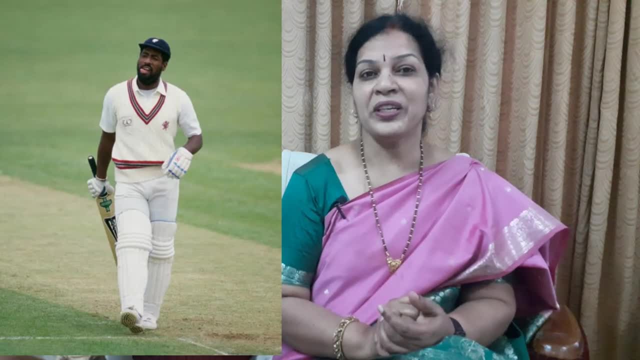 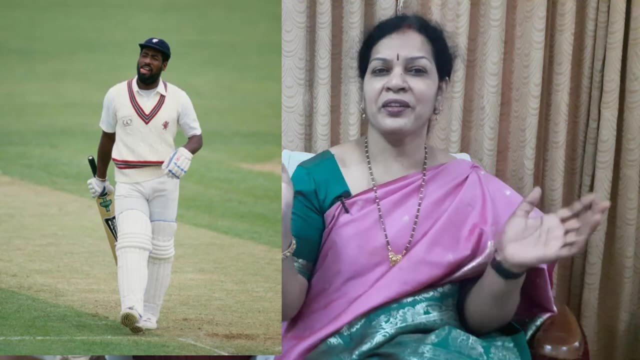 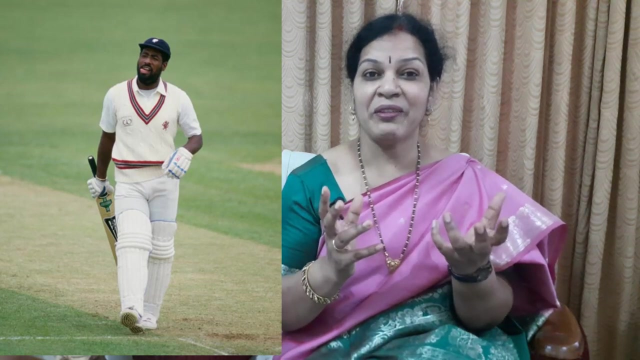 have an idea. so the moment where Vivian Richards used to enter into the ground, he used to chew bubblegum, and also coolly by handling the bat, and had simply coolly used to come. by looking at his attitudes many people used to have a fear. oh, no, fear at all. but if you see him inside, in one of the interviews said: 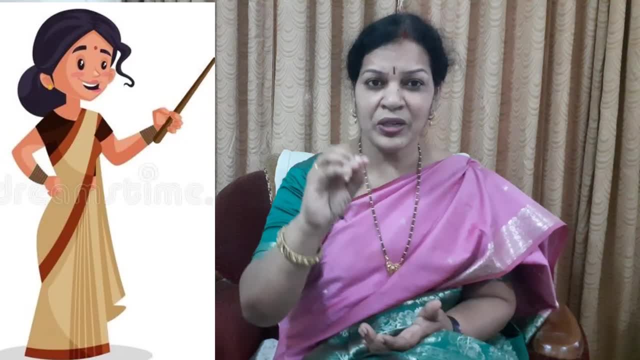 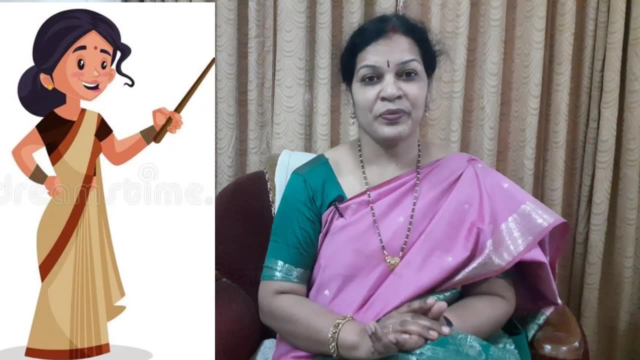 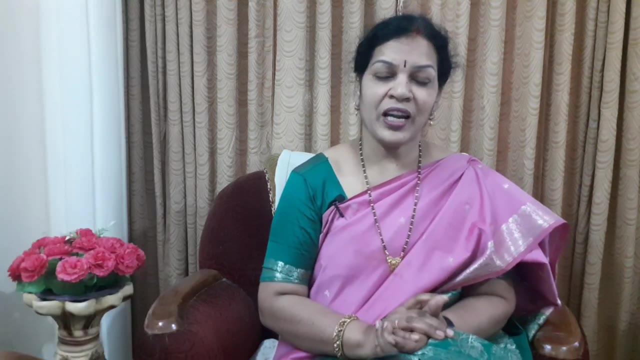 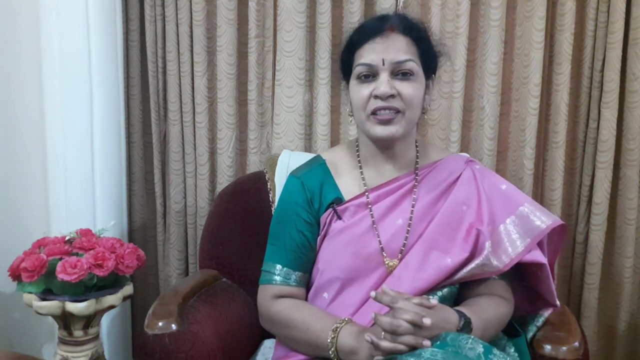 I am telling you They don't know anything. You have to train them. The moment when you feel that they don't know anything, you will not have any fear. And for teaching also, you need to have some practice. Start in front of mirror- or- nowadays technology is there- Record your lectures by yourself and see how you are teaching. how is your body language, how is your communication skills, how you are explaining the concept. 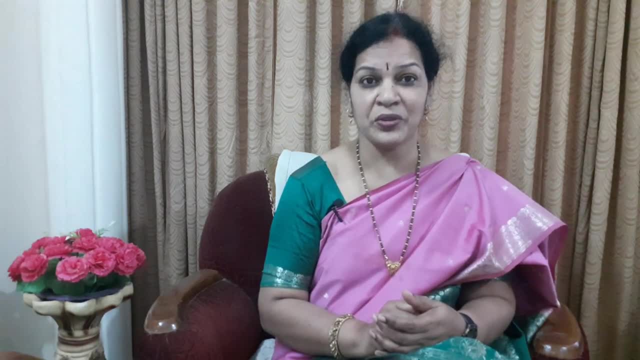 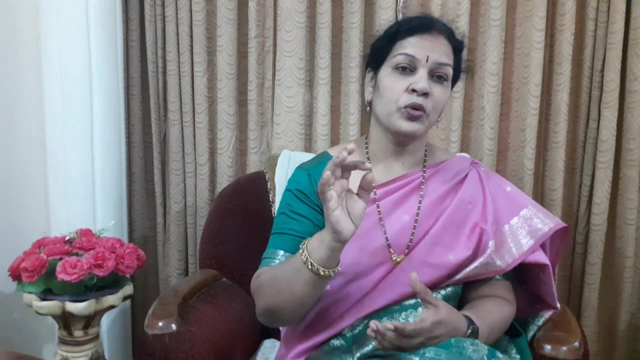 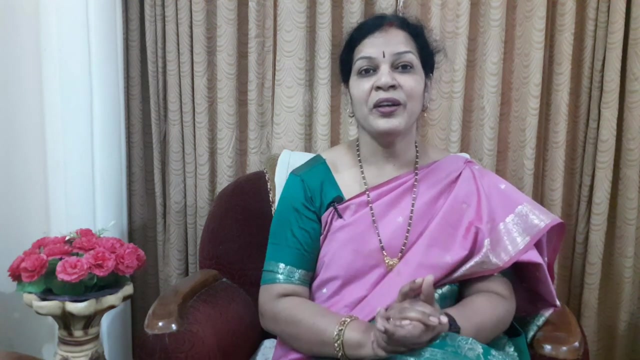 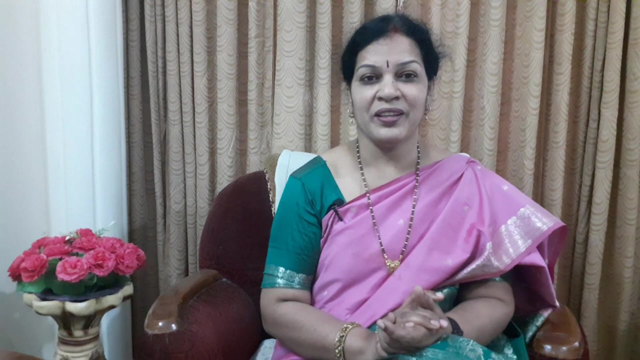 Is it understandable to a common student, average student or below average student? Like you can ask yourself some questions and you can practice it at yourself only. So never have a fear. And the moment when you enter into the class also, please cover that fear with a smiling face. With a smiling face, you can cover that fear. I will tell you the best example In cricket: Vivian Richards from West Indies. 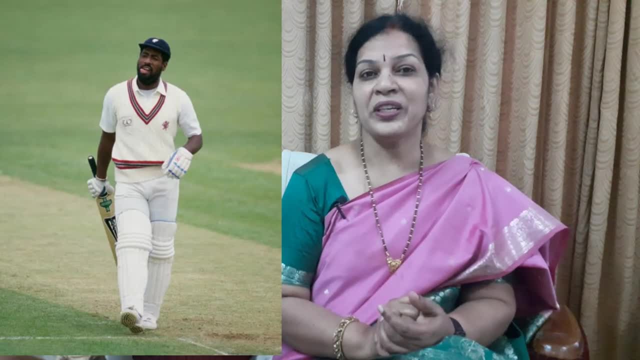 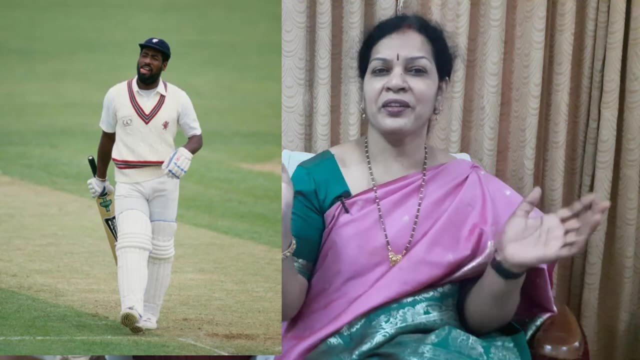 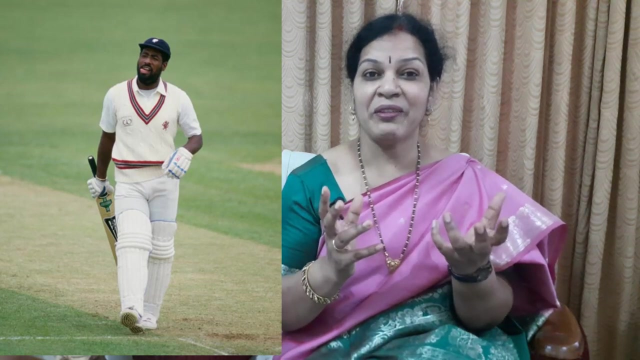 have an idea. so the moment where Vivian Richards used to enter into the ground, he used to chew bubblegum, and also coolly by handling the bat, and had simply coolly used to come. by looking at his attitudes many people used to have a fear. oh, no, fear at all. but if you see him inside, in one of the interviews said: 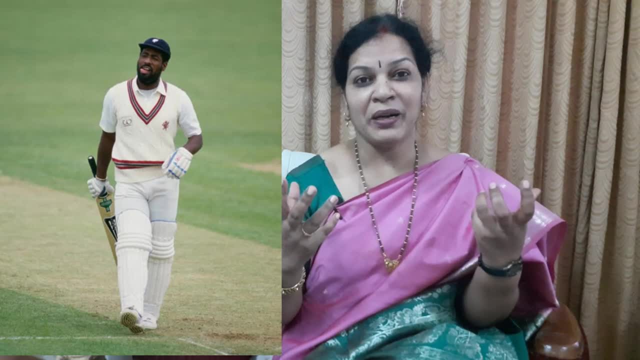 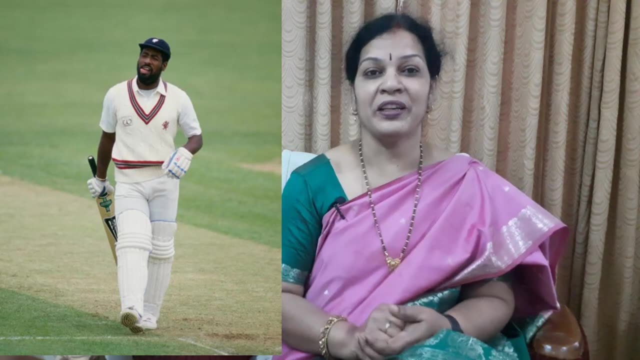 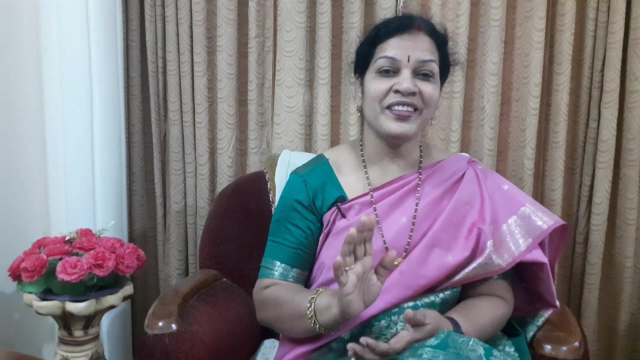 there will be a lot of butterflies inside of my mind, but outside I always express myself cool, so that is going to create a agitation to the opponent party. so in that way, never express your fear to others. be cool, pleasant, cool face and give the confidence to the students that you are going to teach them you are 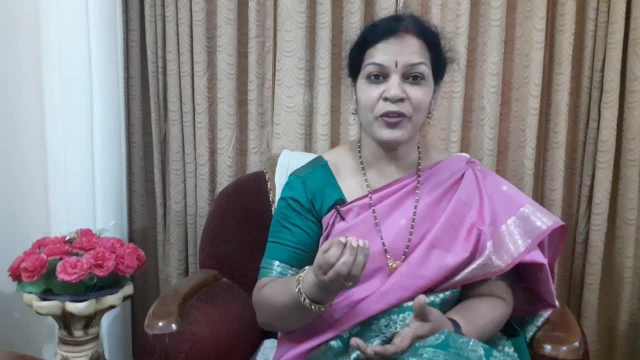 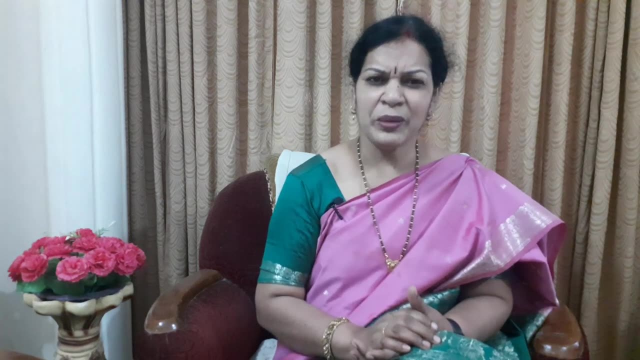 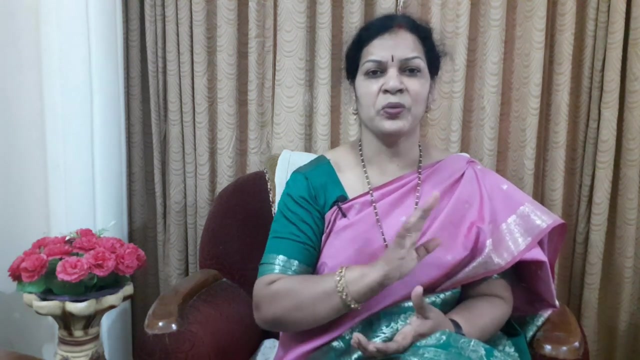 going to do the best of your knowledge. that kind of confidence, that kind of face expressions, you have to keep it so. never have a fear in front of students. sometimes you know that faculty or principal, someone will be sitting inside of the classroom. let them sit, doesn't worry, doesn't matter at all. you are prepared very well, you are. 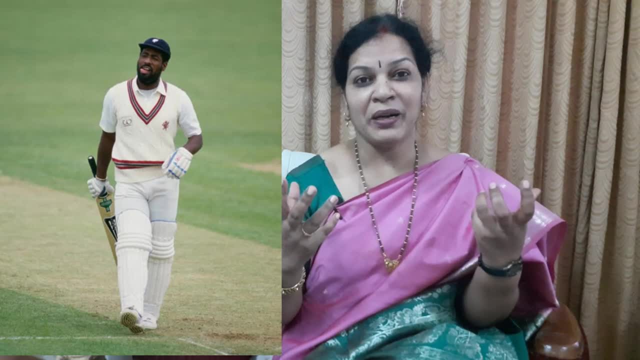 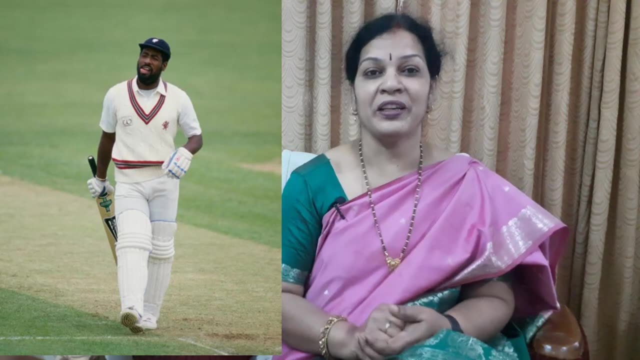 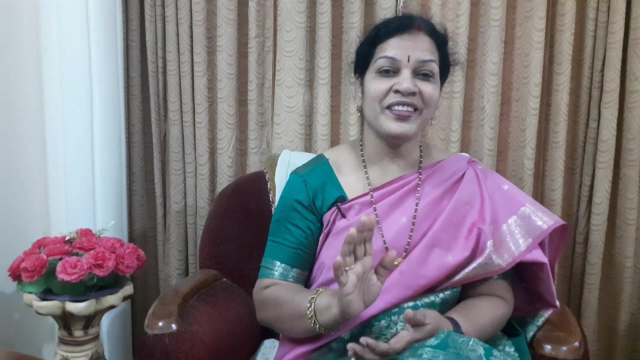 there will be a lot of butterflies inside of my mind, but outside I always express myself cool, so that is going to create a agitation to the opponent party. so in that way, never express your fear to others. be cool, pleasant, cool face and give the confidence to the students that you are going to teach them you are 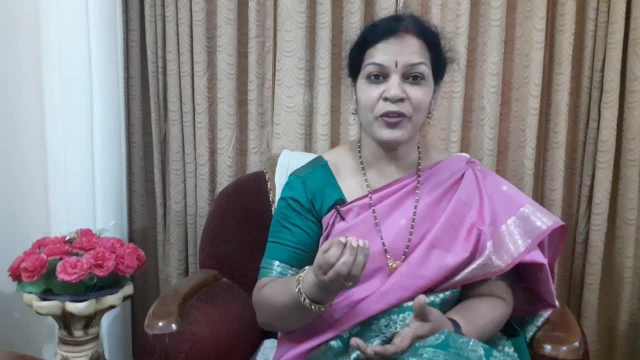 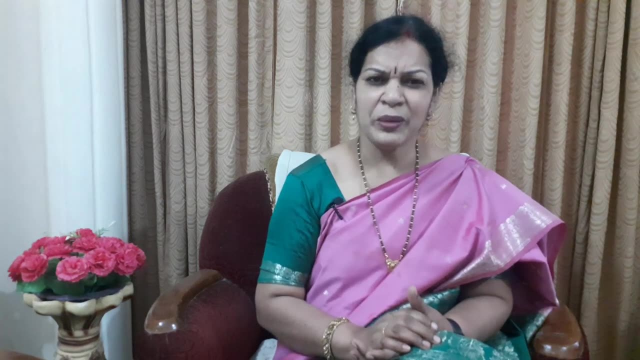 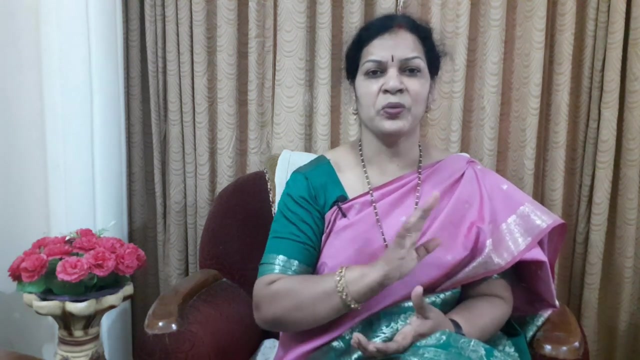 going to do the best of your knowledge. that kind of confidence, that kind of face expressions, you have to keep it so. never have a fear in front of students. sometimes you know that faculty or principal, someone will be sitting inside of the classroom. let them sit, doesn't worry, doesn't matter at all. you are prepared very well, you are. 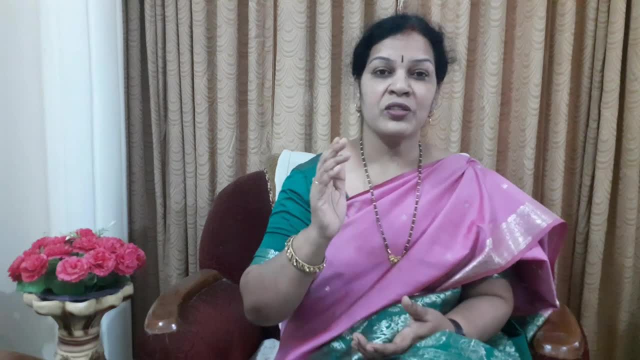 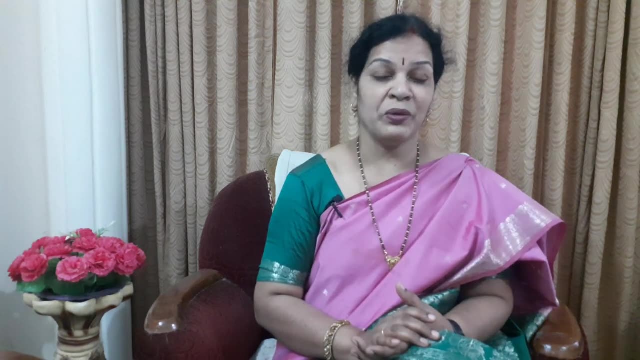 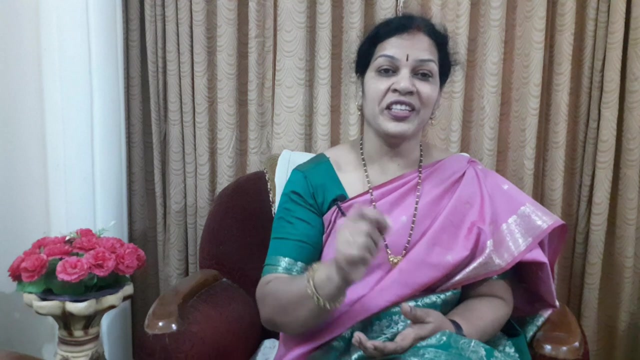 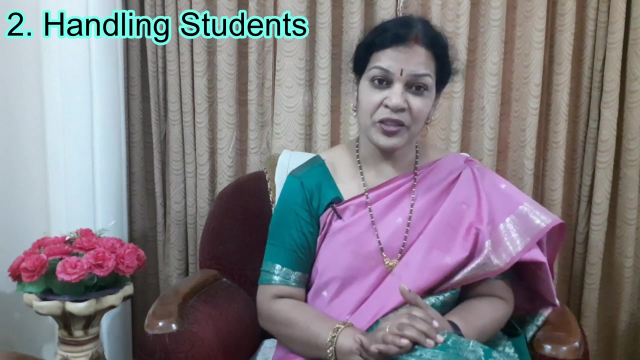 mastered in that subject. so, whatever you know, slowly, coolly express it, ignore those people who are sitting inside of your classroom also, so never have fear about anyone. this is one of the important concept of concept of character of every teacher. second thing is that handling the students, the moment when you go to the classroom, it's a 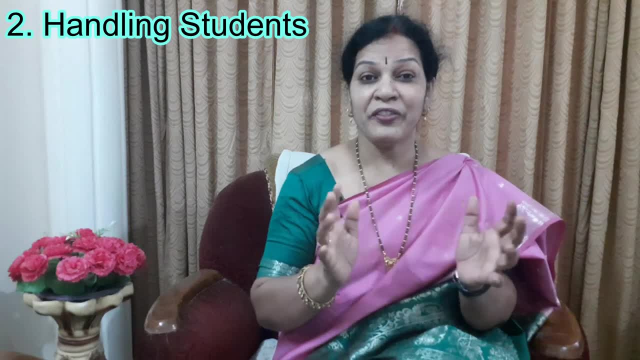 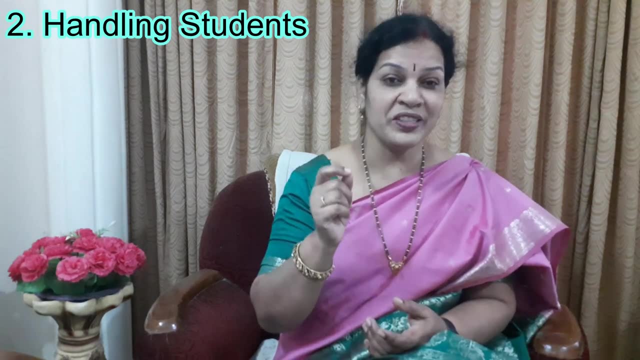 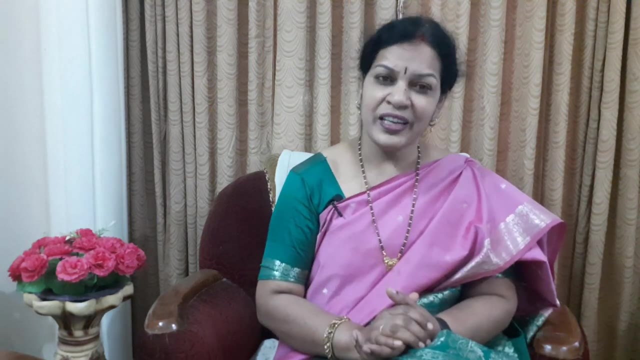 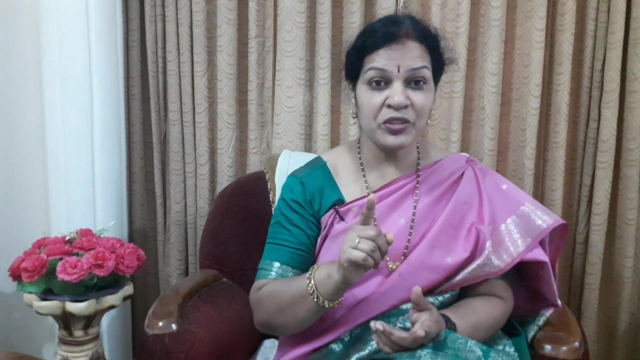 college or school or whatever it may be. you will find different kinds of students. handling these students are very much important. different kinds of students in the sense sometimes you'll find genius students, sometimes average and below average, notorious students, hyperactive students, late Latif means lazy students, so you have to cover up everyone but the moment when you start. 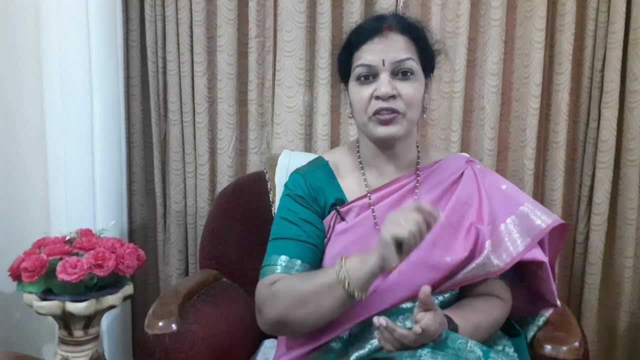 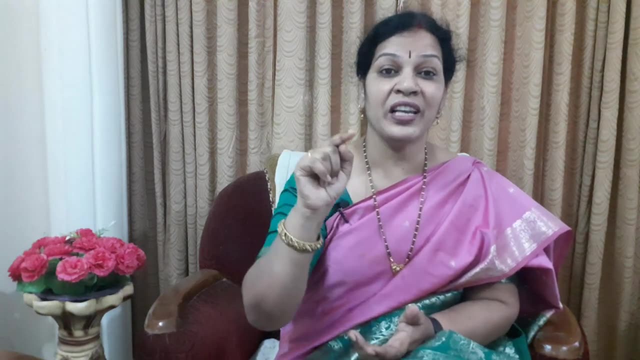 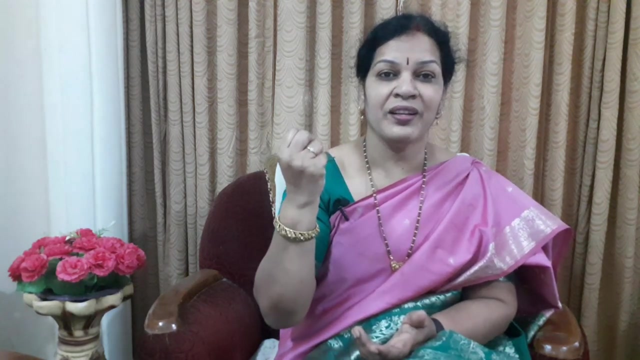 teaching your subject. you have to focus only on the below average student. if that student is able to understand, everyone can understand. from that student point of view, your teaching level should be there. you have to go to their level and teach them and take them, bring them up to your level. that's the. 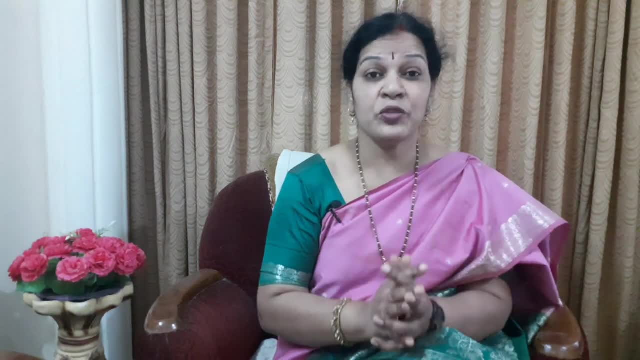 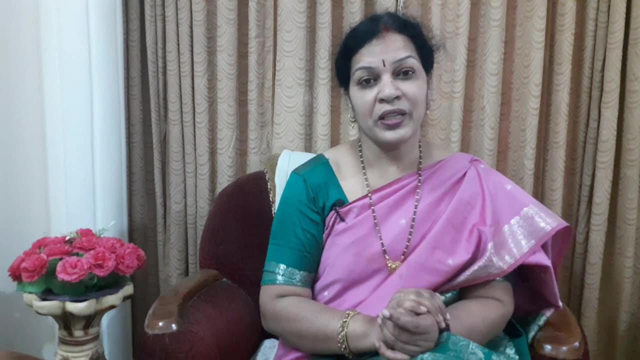 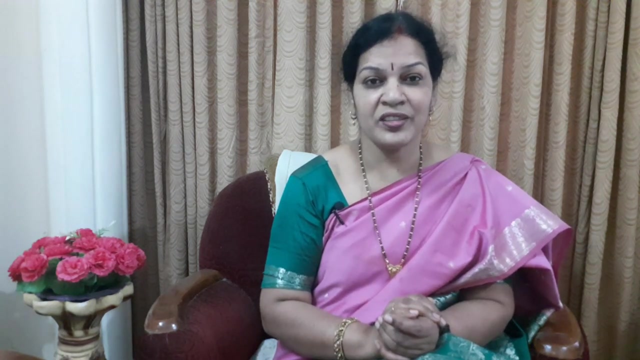 success of every teacher. so, handling these students, notorious, all the students, it comes with your experience. slowly, you, you can understand how to handle, how to talk and how to control them, how to mold these students. all these things slowly you understand, you can just go ahead as per your experience. but 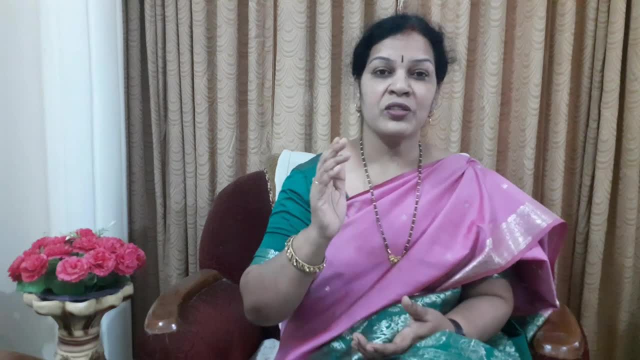 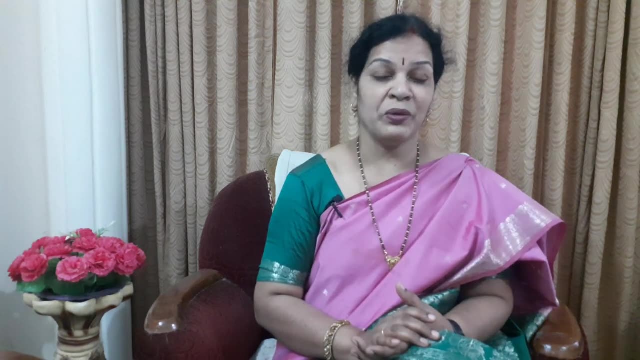 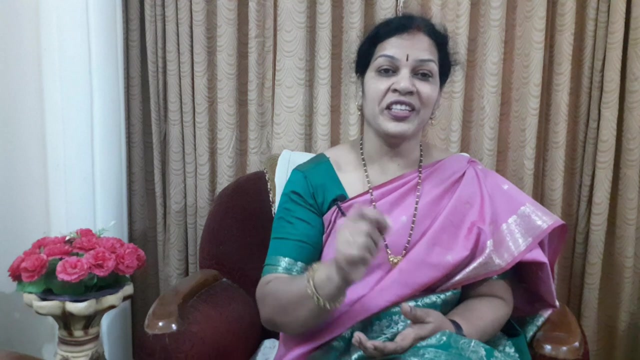 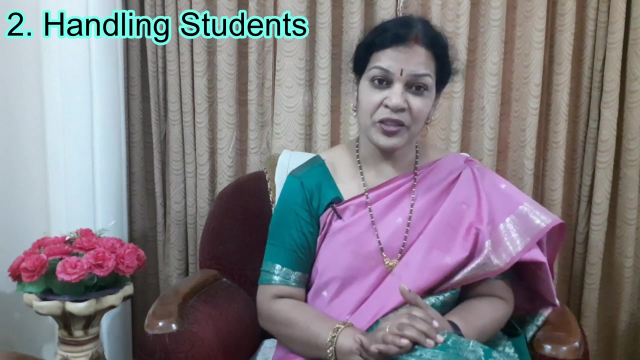 mastered in that subject. so, whatever you know, slowly, coolly express it, ignore those people who are sitting inside of your classroom also, so never have fear about anyone. this is one of the important concept of concept of character of every teacher. second thing is that handling the students, the moment when you go to the classroom, it's a 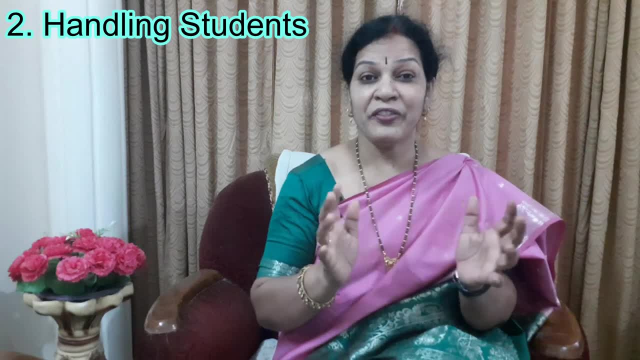 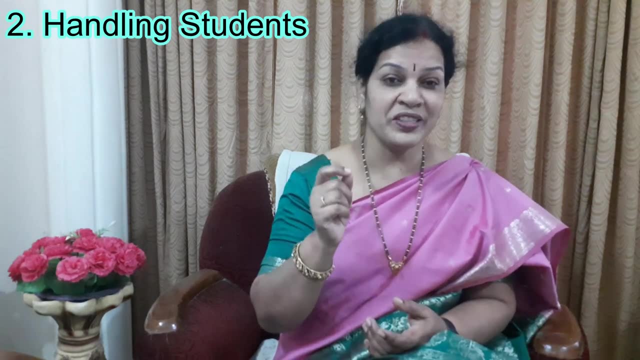 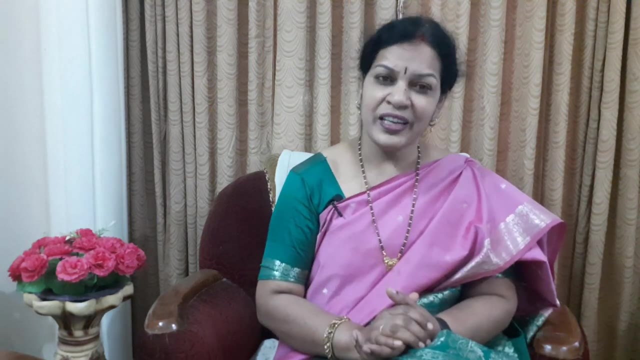 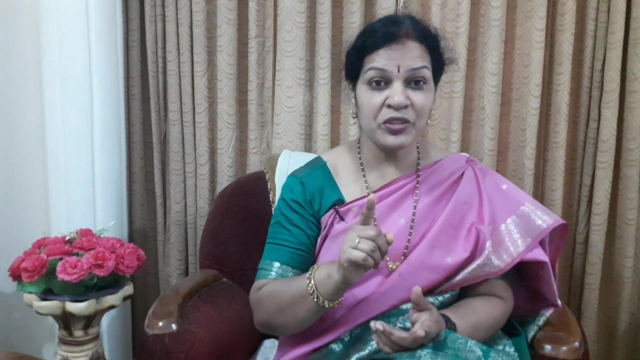 college or school or whatever it may be. you will find different kinds of students. handling these students are very much important. different kinds of students in the sense sometimes you'll find genius students, sometimes average and below average, notorious students, hyperactive students, late Latif means lazy students, so you have to cover up everyone but the moment when you start. 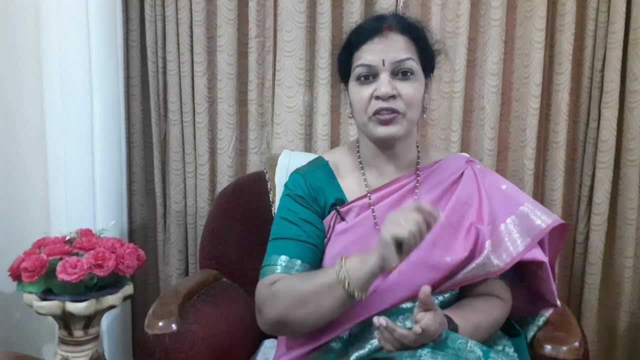 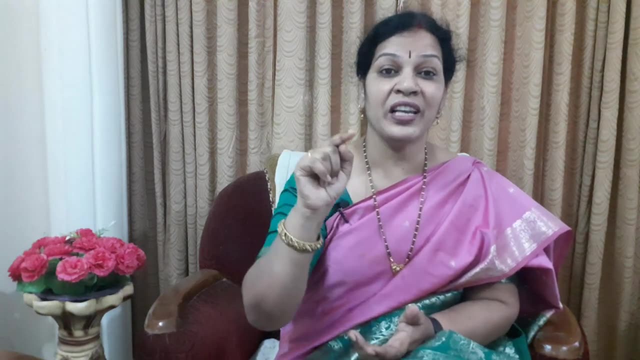 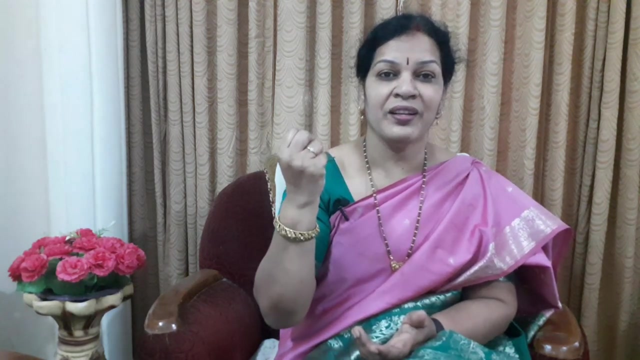 teaching your subject. you have to focus only on the below average student. if that student is able to understand, everyone can understand. from that student point of view, your teaching level should be there. you have to go to their level and teach them and take them, bring them up to your level. that's the. 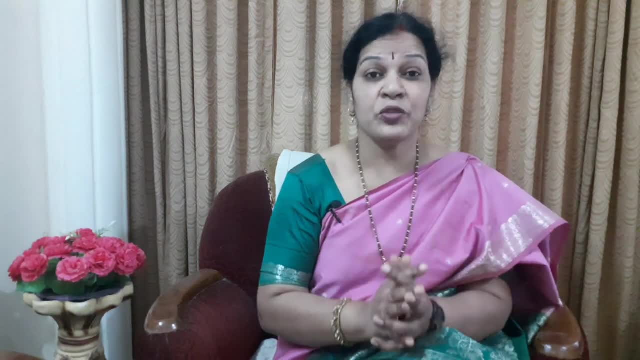 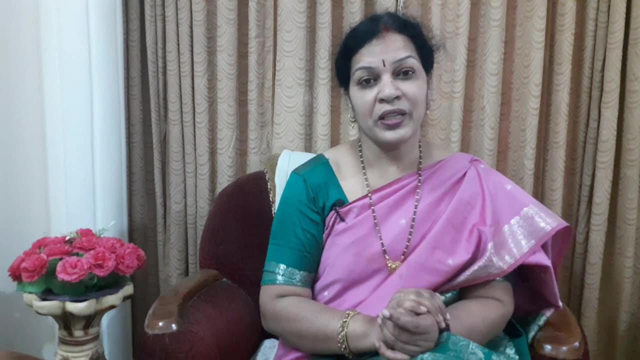 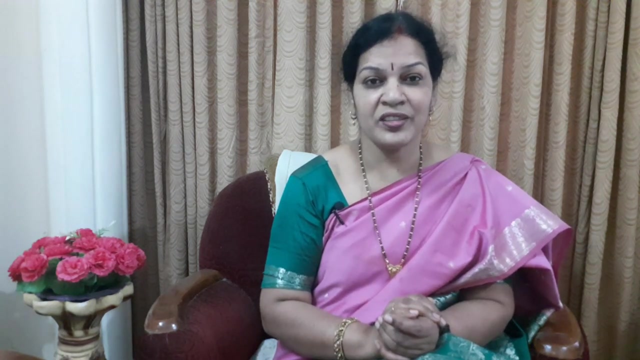 success of every teacher. so, handling these students, notorious, all the students, it comes with your experience. slowly, you, you can understand how to handle, how to talk and how to control them, how to mold these students. all these things slowly you understand, you can just go ahead as per your experience. but 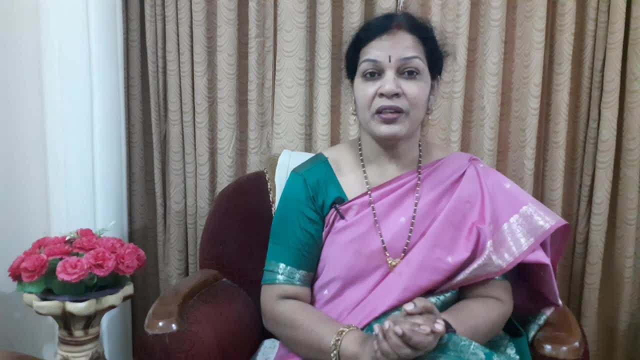 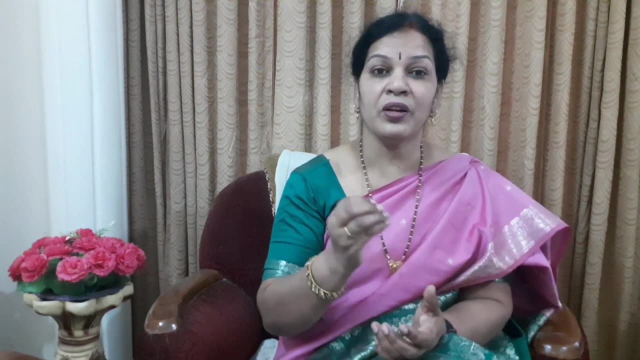 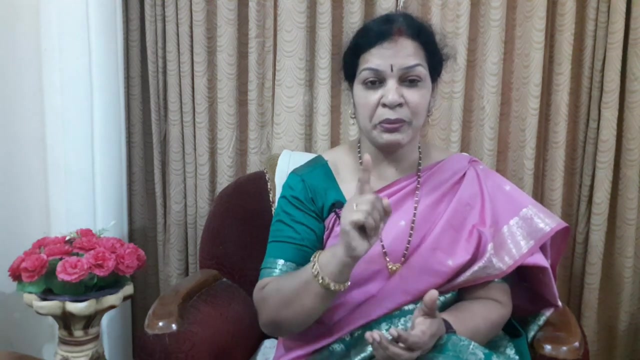 never be hyperactive or others. never take any kind of temptations angry and showing your anger on students. this kind of things don't do always. the teacher should- should have a lot of patience. patience is one of the best quality of every teacher. please remember this point. 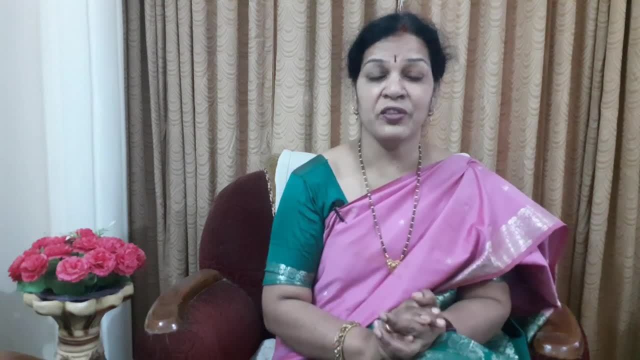 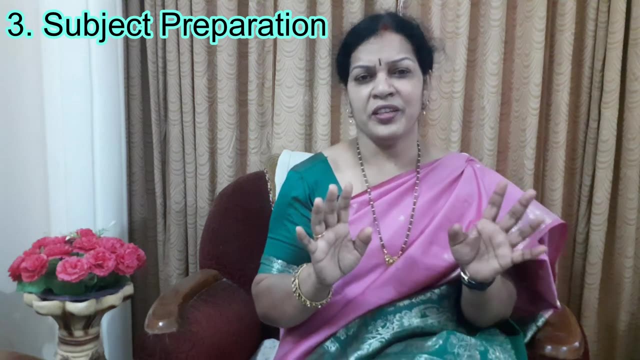 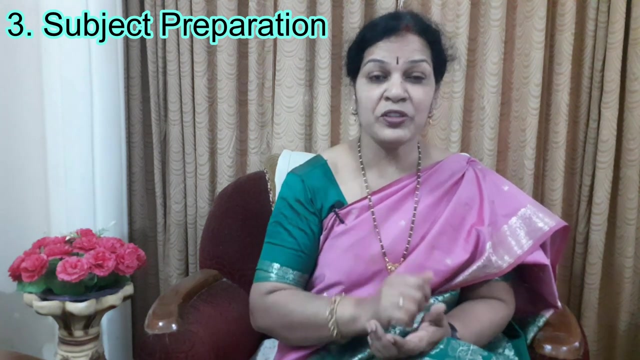 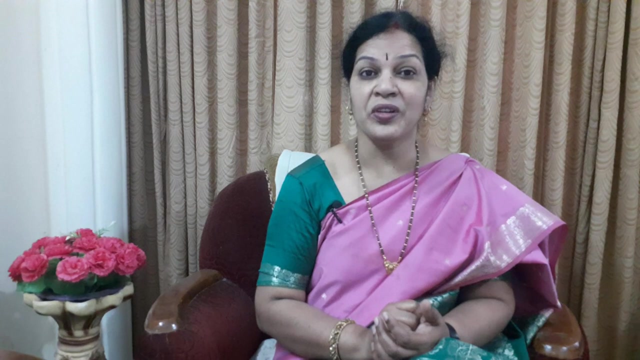 so handling the students is must, must learn for all the teachers. and third one, third one is that subject preparation. there is no alternative, there is no substitute than the subject knowledge. unless you have a very good command over subject you can't attract any student. no student will like a teacher who is not. 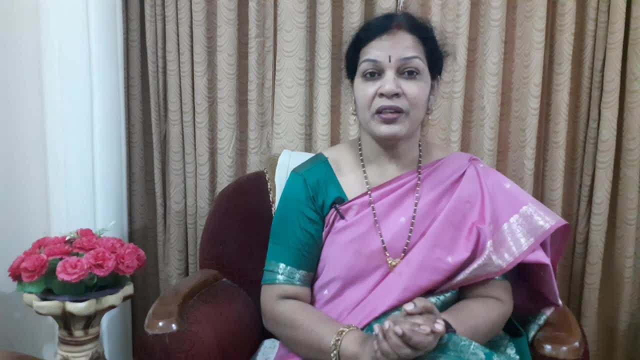 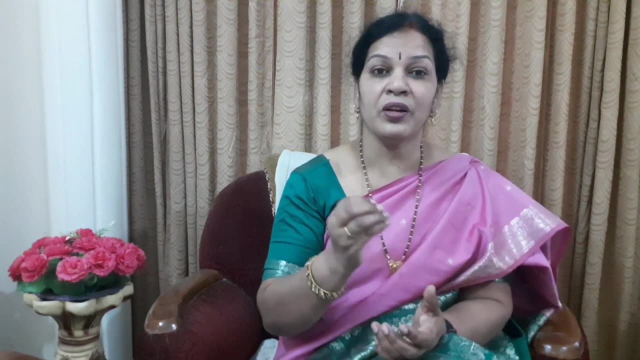 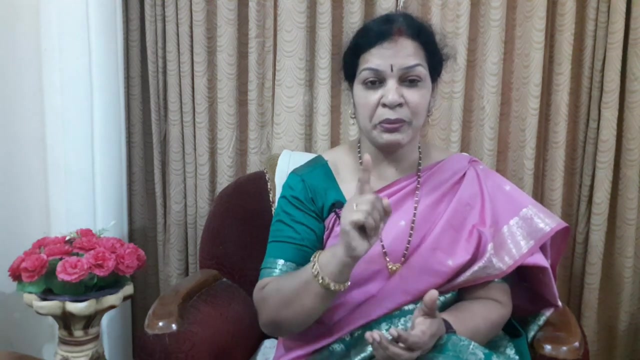 never be hyperactive or others. never take any kind of temptations angry and showing your anger on students. this kind of things don't do always. the teacher should- should have a lot of patience. patience is one of the best quality of every teacher. please remember this point. 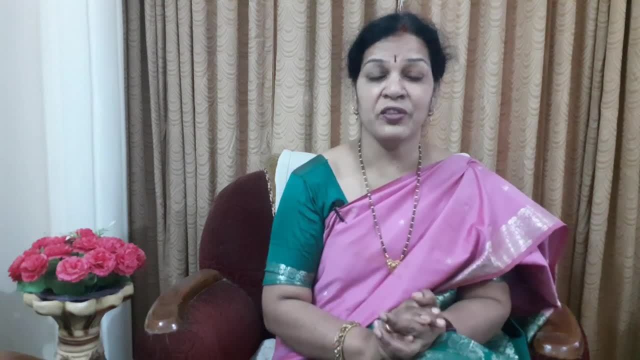 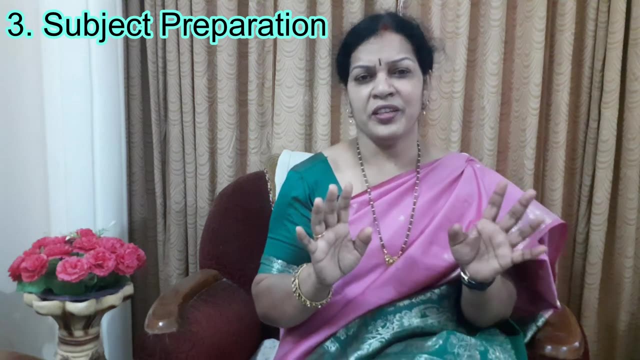 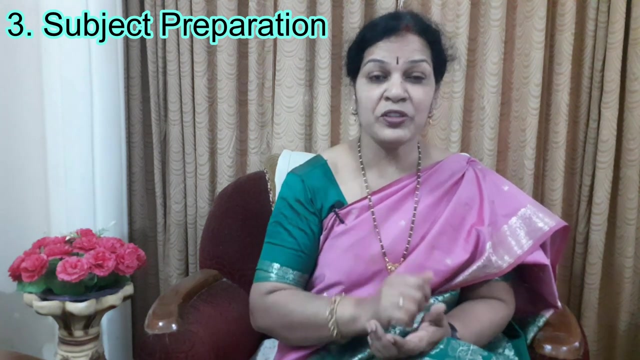 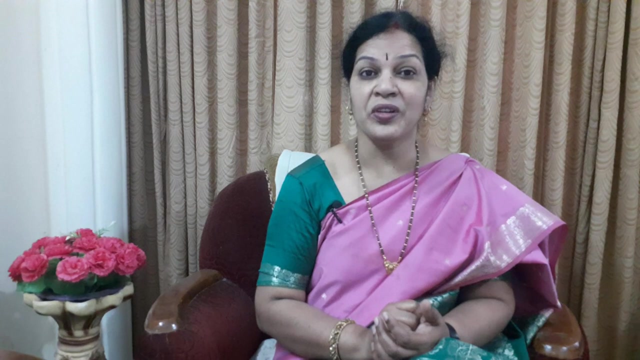 so handling the students is must, must learn for all the teachers. and third one, third one is that subject preparation. there is no alternative, there is no substitute than the subject knowledge. unless you have a very good command over subject you can't attract any student. no student will like a teacher who is not. 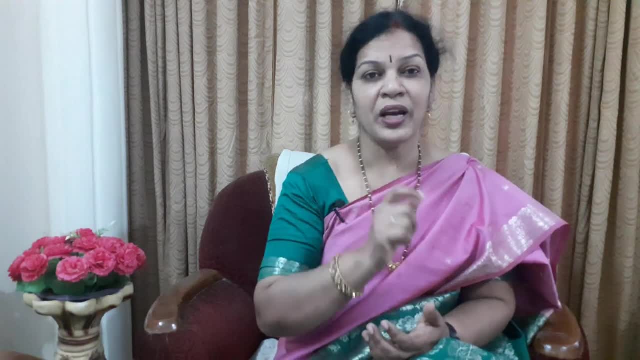 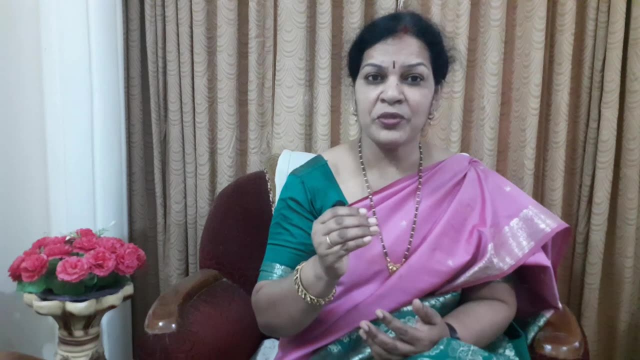 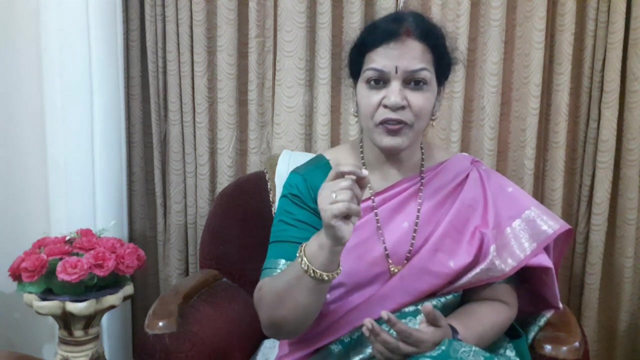 having command over the subject. so that is why you need to have the command over that topic and go with a lot of thorough preparation, and when you prepare the subject you know that I'll tell you the attitude when you prepare the subject, study for you are sick. understand for yourself. then after that, once, if you get, 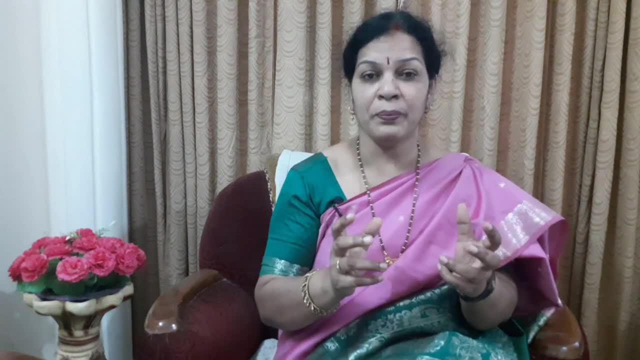 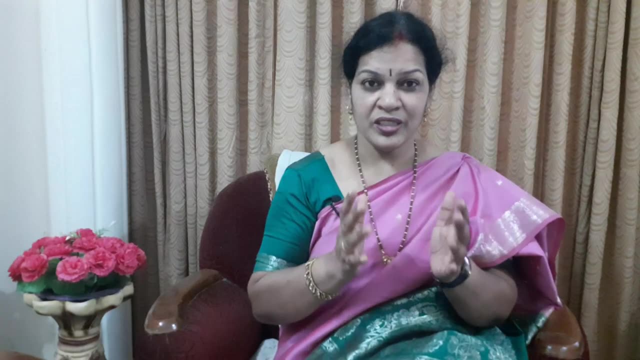 a command once. if you understand once, if you are thorough with the top topic, then think about how to explain, how to explain to the students. so this is very important thing. you can observe something and then you can learn how to explain to the students. so this is very important thing you can observe. 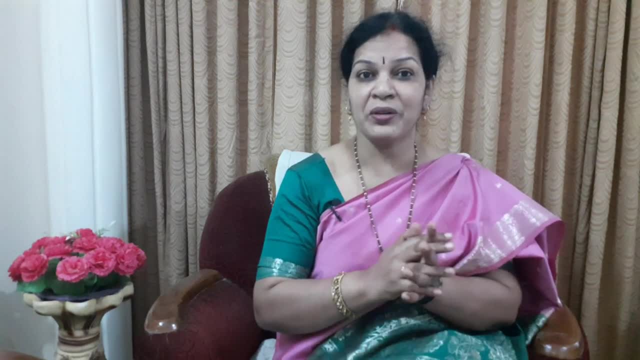 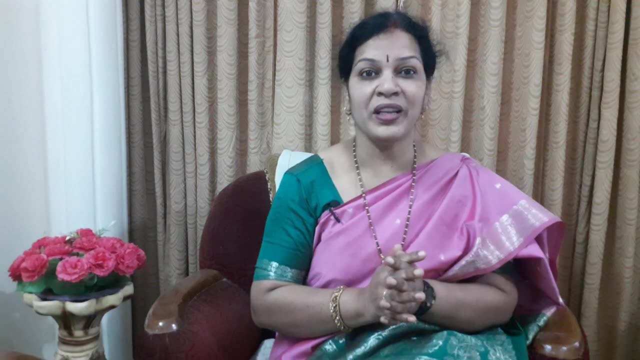 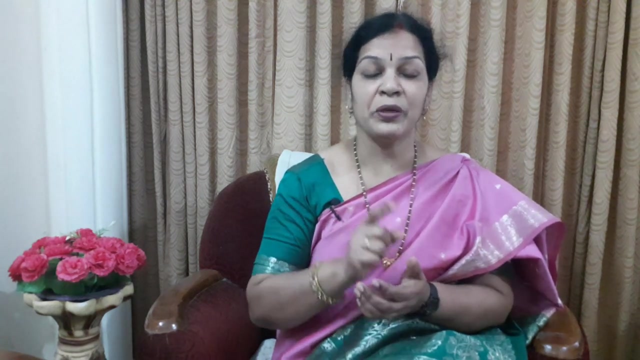 some of your previous teachers who taught you at school level- college level, who was your favorite teacher? also you can observe, you can just recollect how they used to teach. how was the body language, their teaching style, communication skills, mannerism, all these things you can just recollect it. but 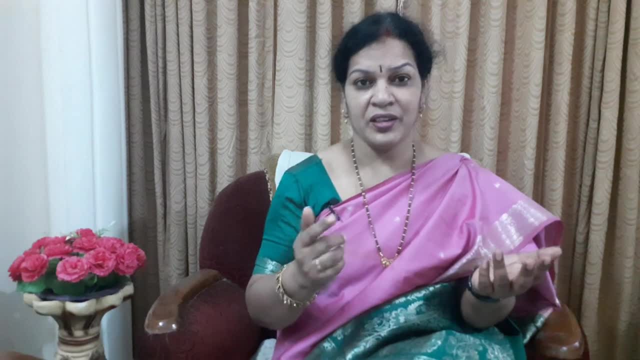 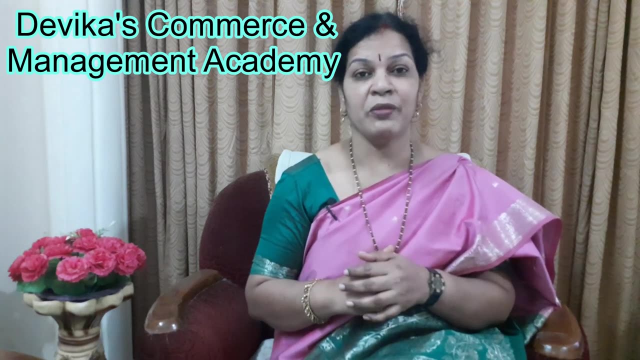 don't copy anyone. you should have your own style. you can observe some of my lectures in Davy course, commerce and management Academy. so in this sub, in this channel, I've been teaching many subjects related to the commerce and management, so you can observe how I was teaching. 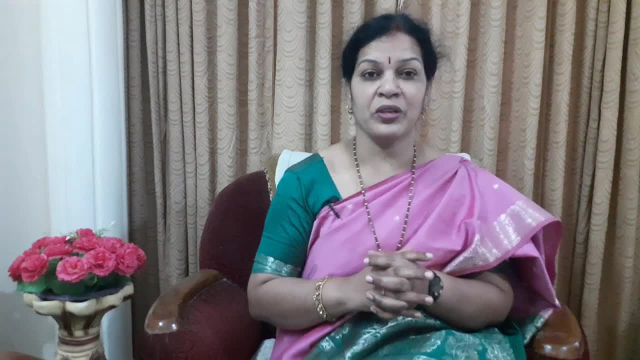 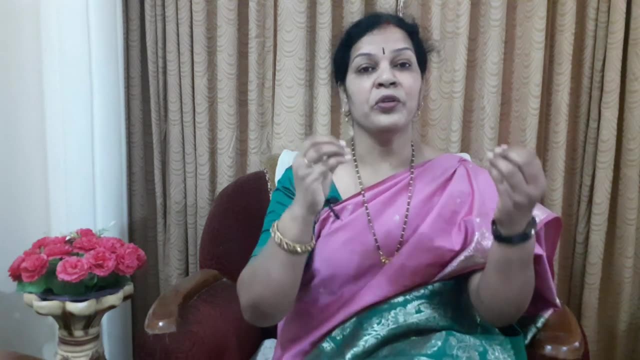 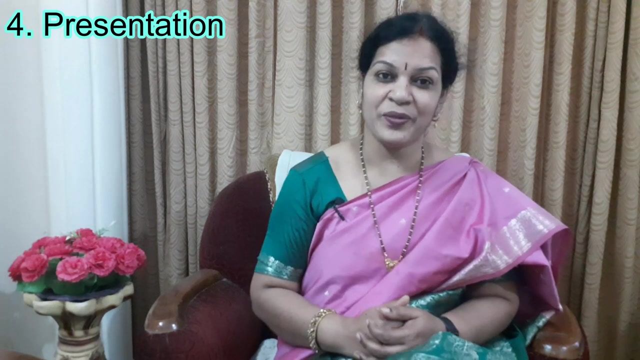 and how is my style and all these things also. you can observe it. so that is why subject preparation is important. your, your thoroughness and how you are going to present it. that is important. and fourth point is that presentation, how do you present yourself? your presentation is important, presentation in the sense. 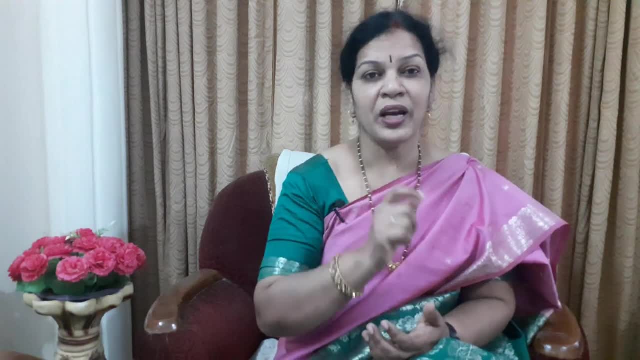 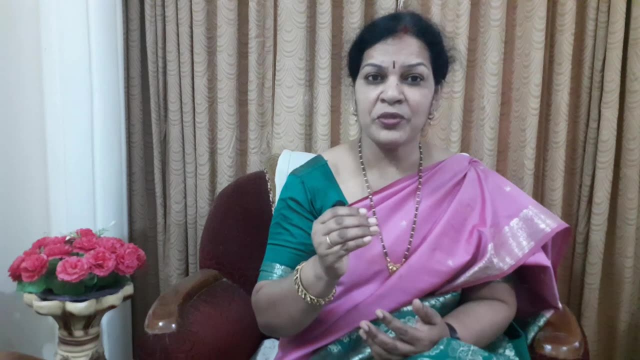 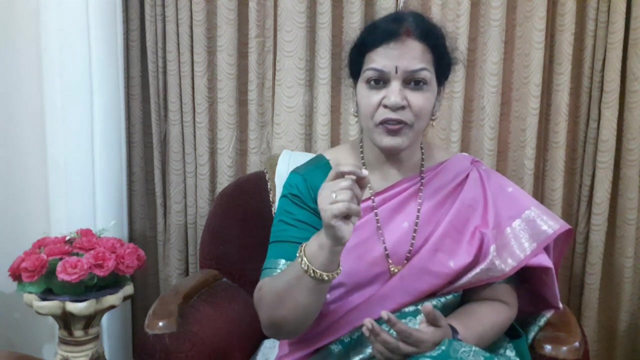 having command over the subject. so that is why you need to have the command over that topic and go with a lot of thorough preparation, and when you prepare the subject you know that I'll tell you the attitude when you prepare the subject, study for you are sick. understand for yourself. then after that, once, if you get, 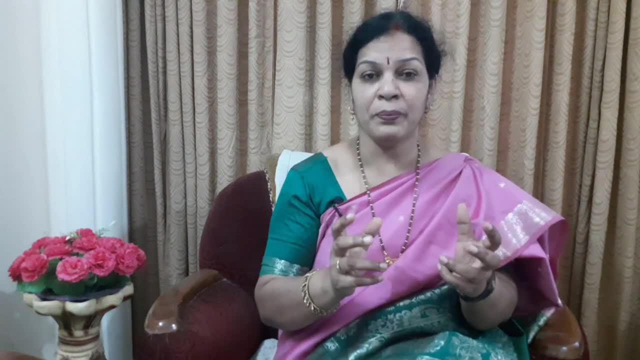 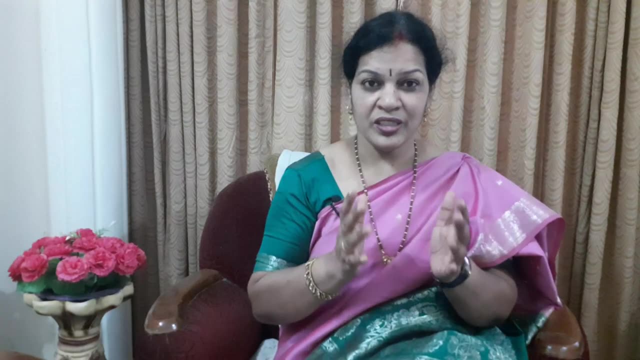 a command once. if you understand once, if you are thorough with the top topic, then think about how to explain, how to explain to the students. so this is very important thing. you can observe something and then you can learn how to explain to the students. so this is very important thing you can observe. 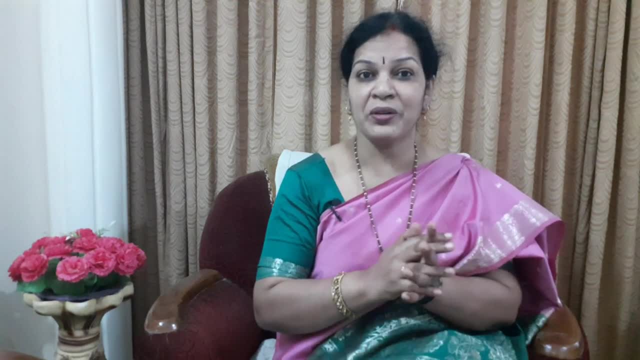 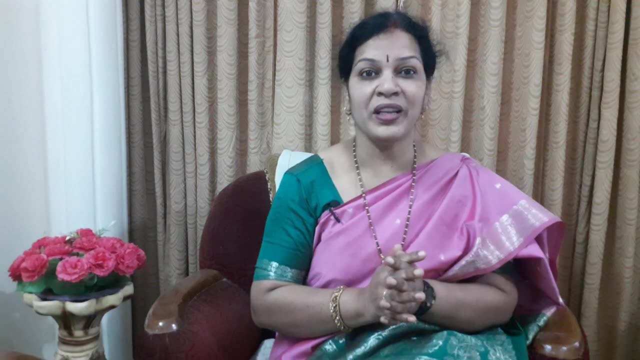 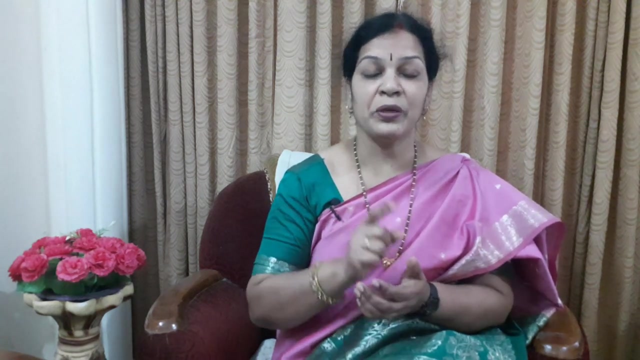 some of your previous teachers who taught you at school level- college level, who was your favorite teacher? also you can observe, you can just recollect how they used to teach. how was the body language, their teaching style, communication skills, mannerism, all these things you can just recollect it. but 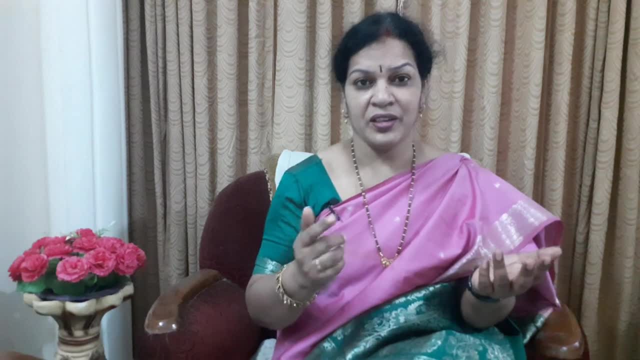 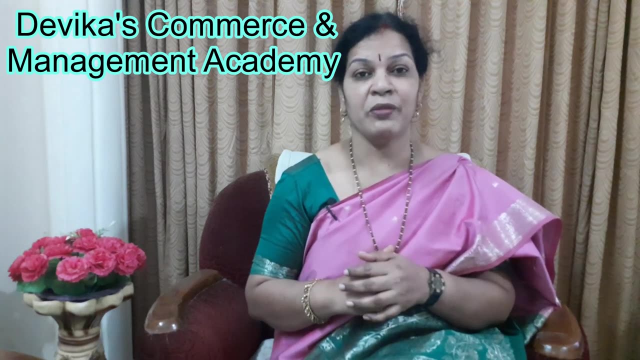 don't copy anyone. you should have your own style. you can observe some of my lectures in Davy course, commerce and management Academy. so in this sub, in this channel, I've been teaching many subjects related to the commerce and management, so you can observe how I was teaching. 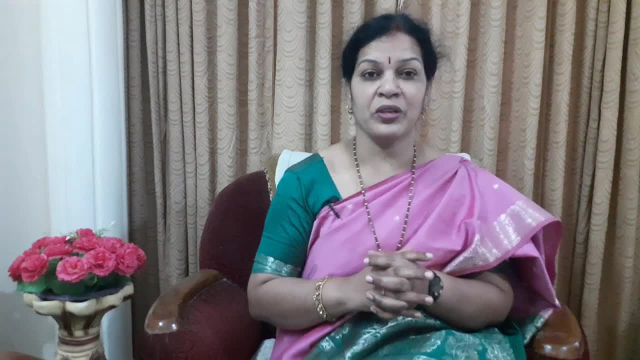 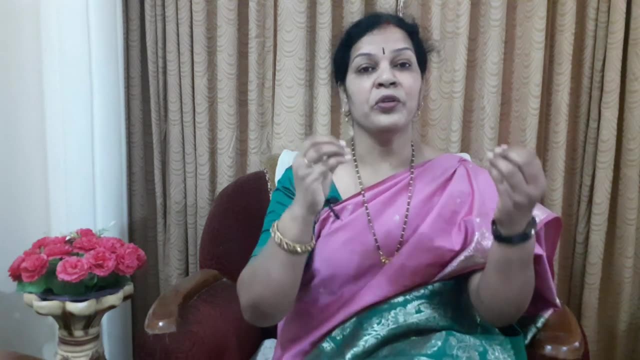 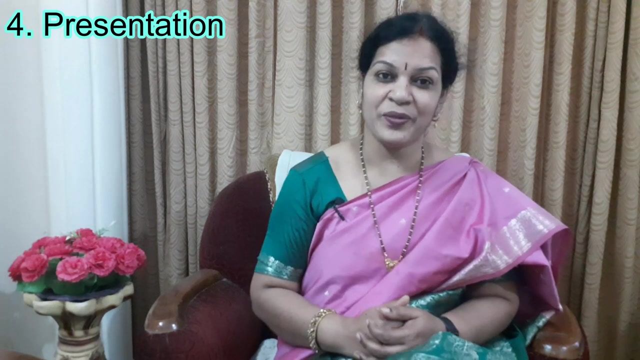 and how is my style and all these things also. you can observe it. so that is why subject preparation is important. your, your thoroughness and how you are going to present it. that is important. and fourth point is that presentation, how do you present yourself? your presentation is important, presentation in the sense. 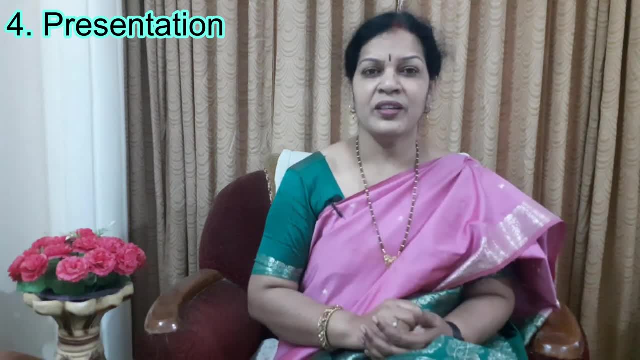 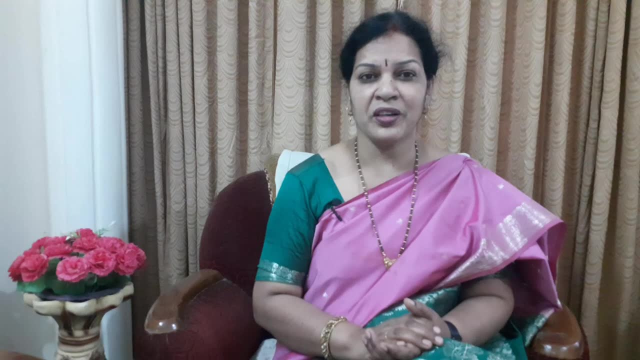 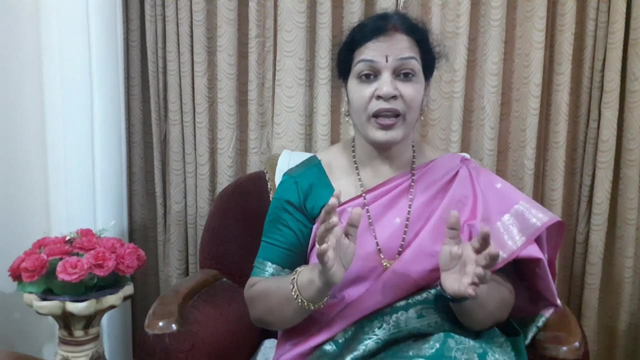 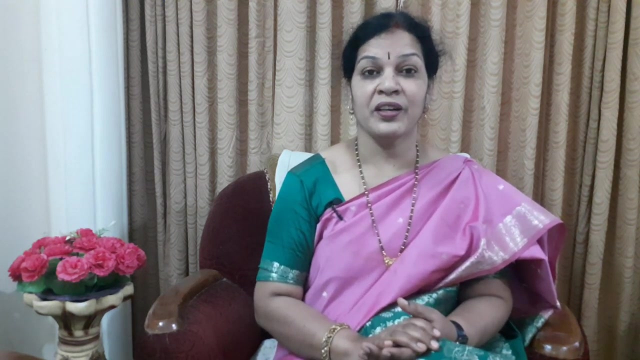 only two things comes over here. one is having a command over the communication skills. communication skills in the sense need not to use any jargon words and confusing the students not required. just speak slowly, coolly, comfortably, where an average student can understand your language in that way. use your language coolly. speak communication skills okay. 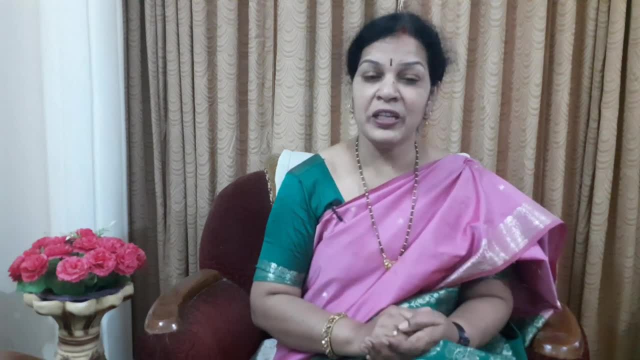 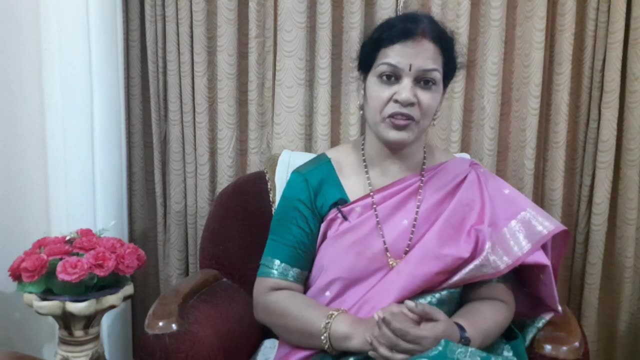 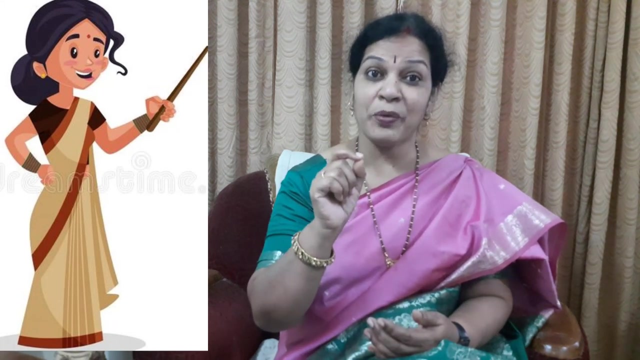 and also, if your communication skills are not good, please improve it, practice it. the more you practice it, you'll get more command over your communication skills and also body language. the moment when a teacher enters inside of the classroom, the students looks at the appearance and body language of a teacher. if body language 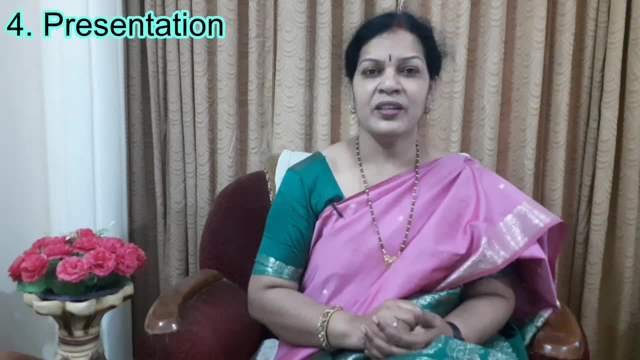 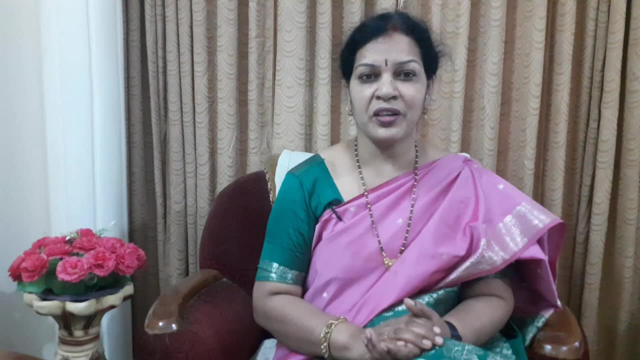 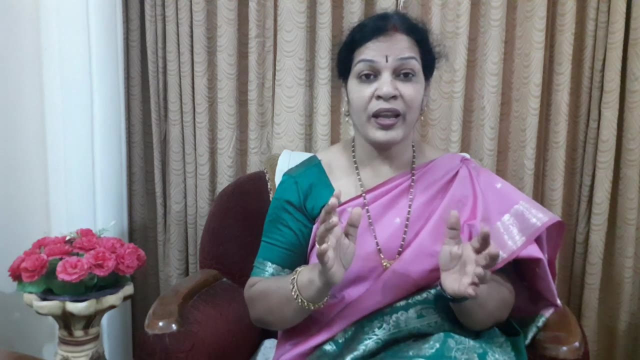 only two things comes over here. one is having a command over the communication skills. communication skills in the sense need not to use any jargon, words on confusing. it's not required just to speak slowly, coolly, comfortably, where an average student can understand your language in that way. use your language, cool, speak. 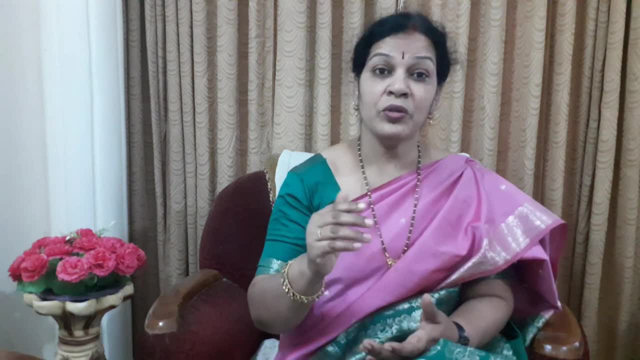 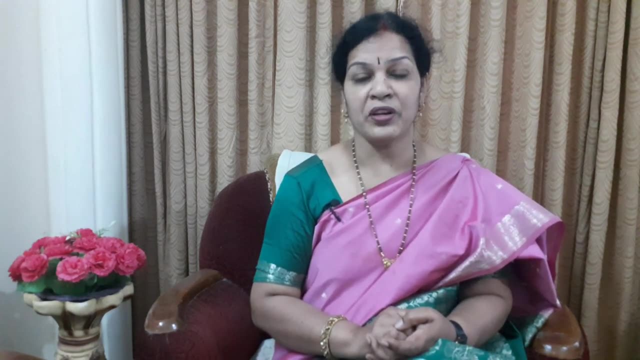 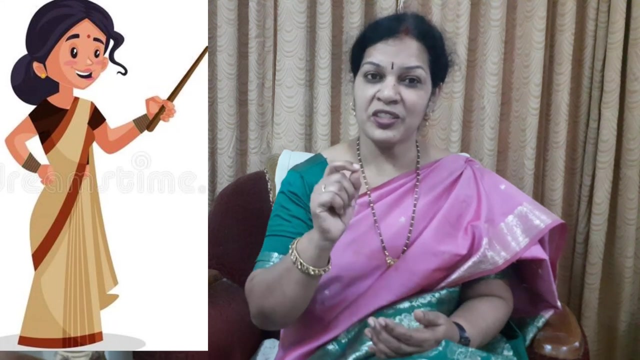 communication skills okay. and also, if your communication skills are not good, please improve it, practice it. the more you practice it, you'll get more command over it- your communication skills and also body language. the moment when a teacher enters inside of the classroom, the students looks at the appearance and body language of a teacher. if body language 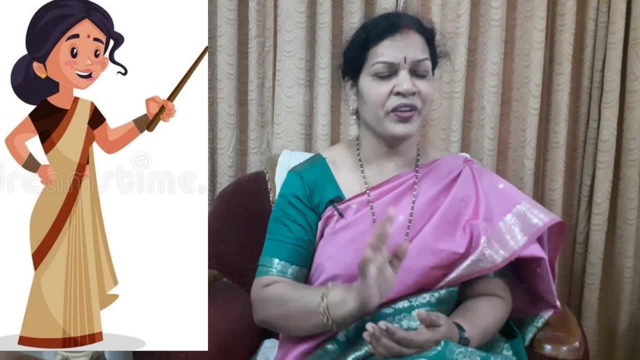 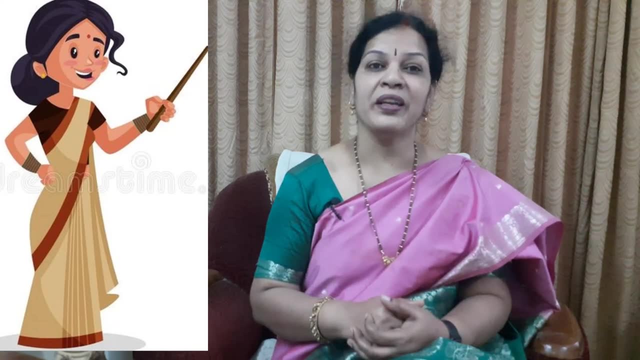 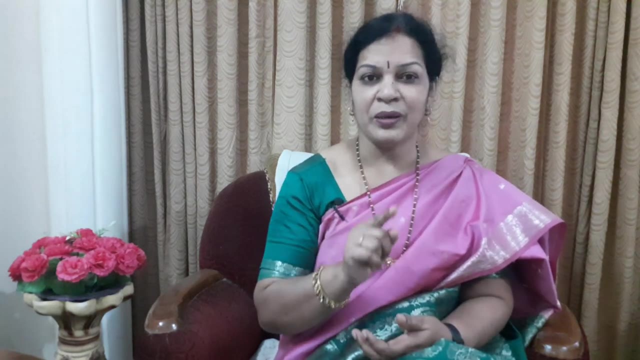 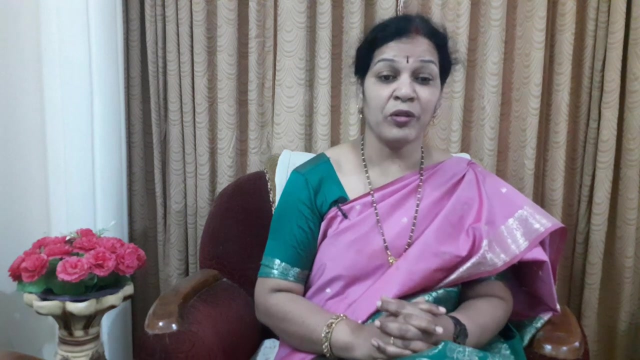 is cool, pleasant and giving a confidence, then automatically the students will get a lot of confidence. 50 percent of the students will be getting attracted by the body language and communication skill of any teacher. so that is why please be careful about a good communication skills and a pleasant body language. and fifth point I would like to say is attitude and also. 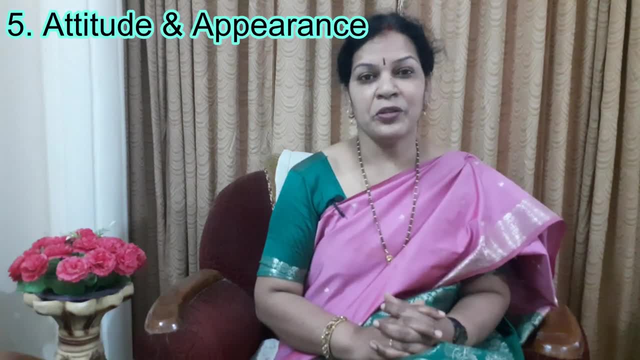 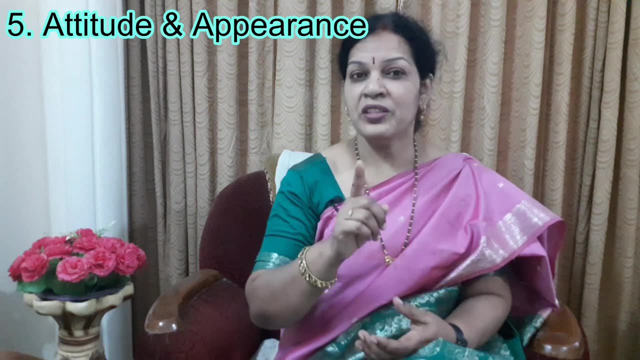 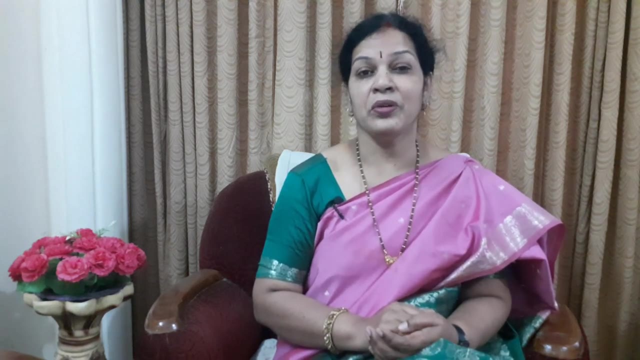 appearance. you know that some of the teachers attitude will be very rough and tough, very hard, and ego feelings will be there. students will never accept that kind of teachers and they won't understand that lecture. also, they won't get good marks. there will be no attachment with that teacher. that is why 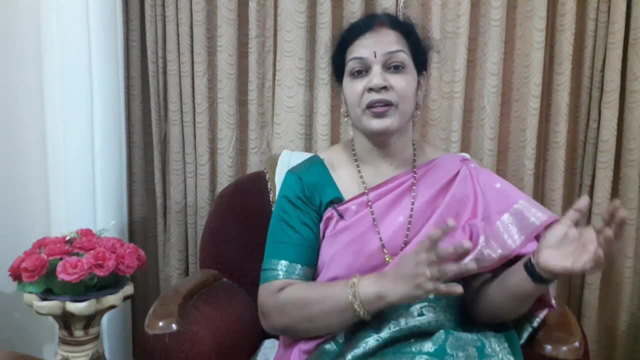 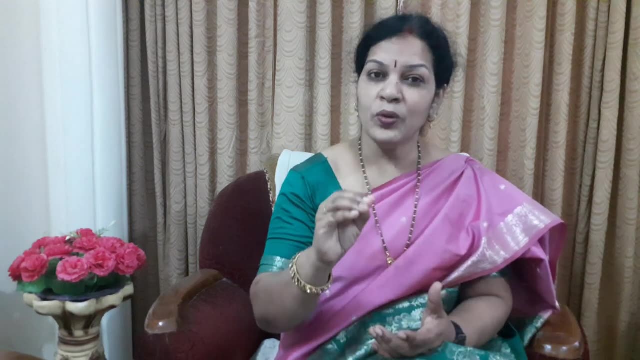 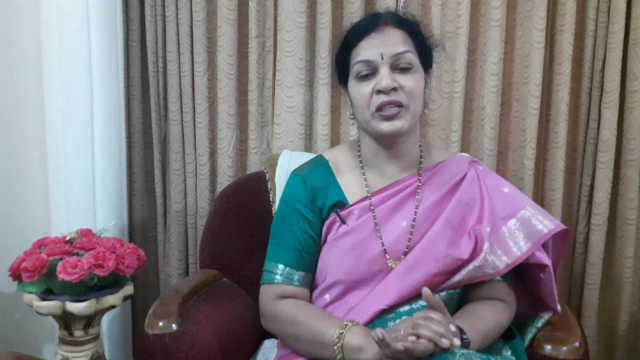 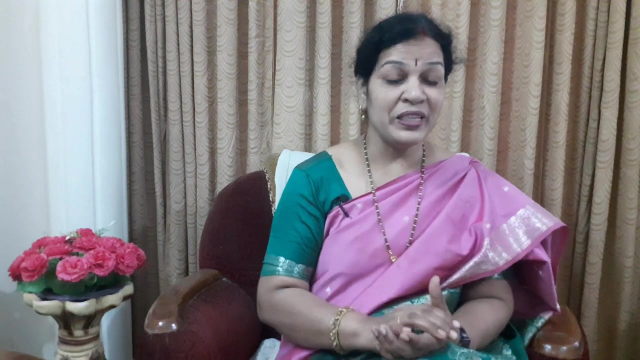 always keep your ego rough and very hard nature and all these things keep it aside. always be cool and give them a confidence that whatever you are going to teach the students are going to understand. that kind of assurance to give it to them, then automatically students will start loving your lectures. and always pleasing face is important if 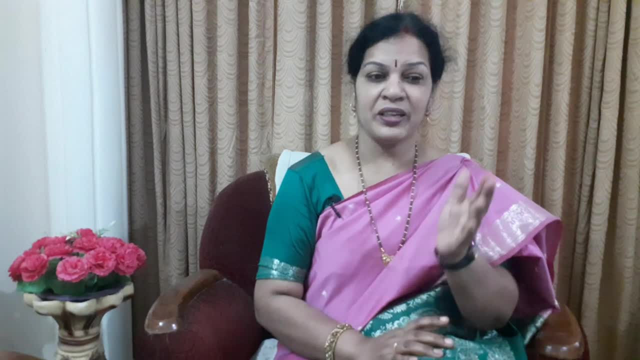 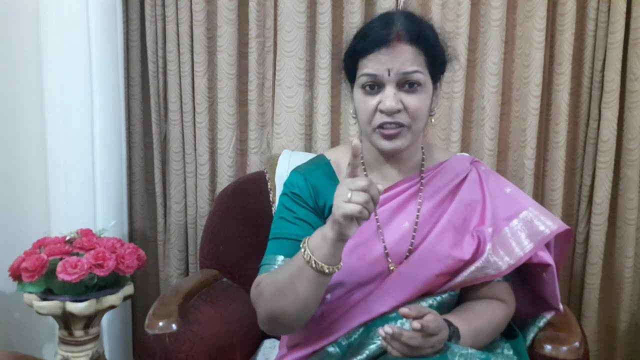 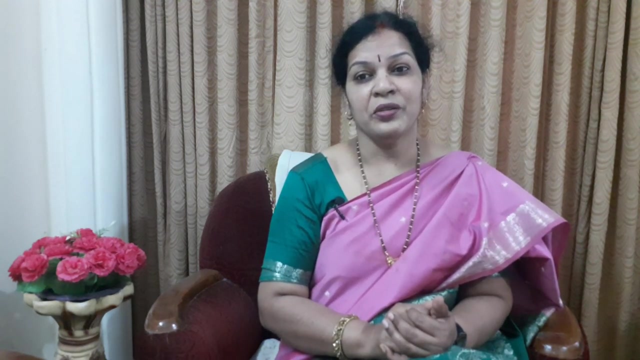 in that way you keep it and, at the same time, your attitude along with attitude, appearance- appearance also matters a lot, especially young teachers are telling you, whatever may be your age, just a completed post graduation and your age is maybe 22, 23, whatever may be your age, you. 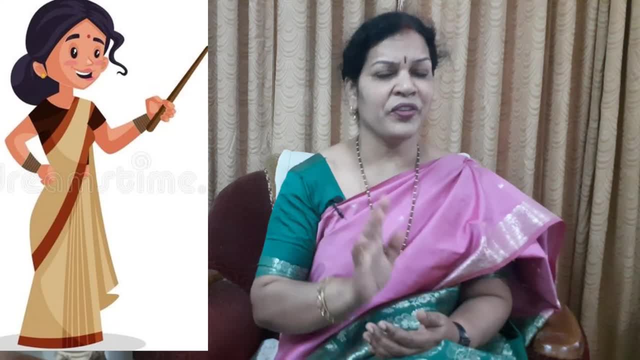 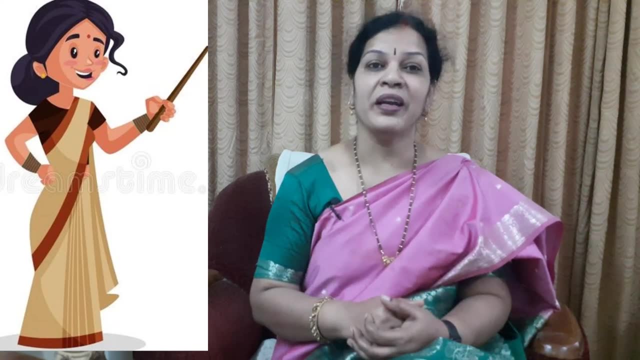 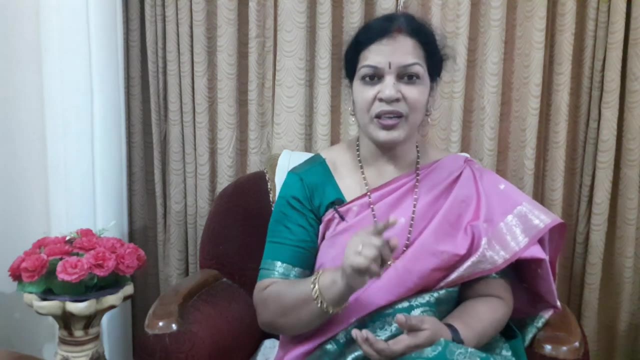 is cool, pleasant and giving a confidence, then automatically the students will get a lot of confidence. fifty percent of the students will be getting attracted by the body language and communication skill of any teacher. so that is why please be careful about a good communication skills and a pleasant body language. and fifth point I would like to say is attitude. 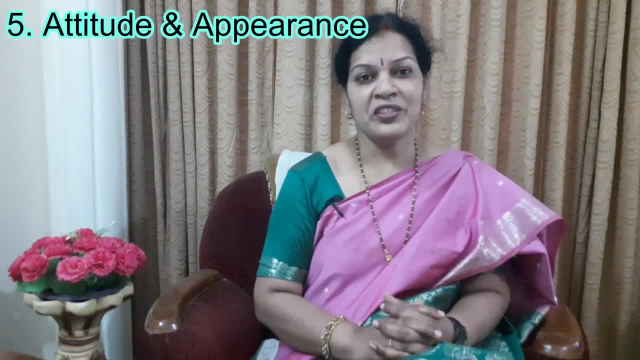 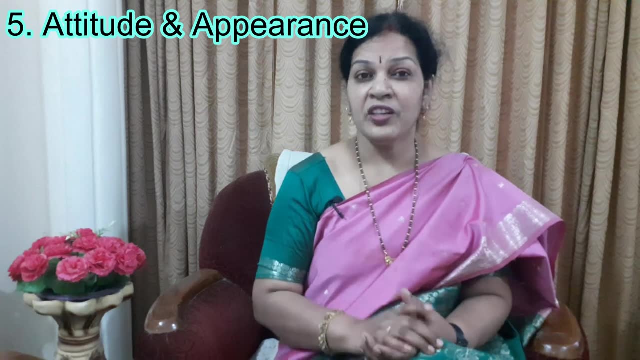 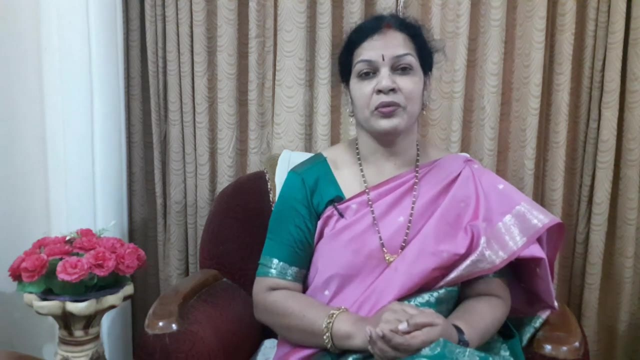 and also appearance. you know that some of the teachers attitude will be very rough and tough, very hard, and ego feelings will be there. students will never accept that kind of teachers and they won't understand that lecture. also, they won't get good marks. there will be no attachment with that teacher. that is why always 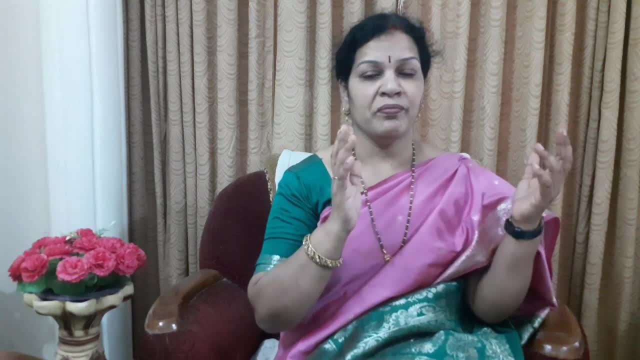 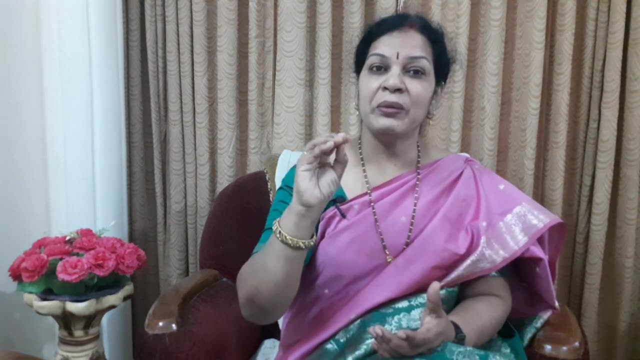 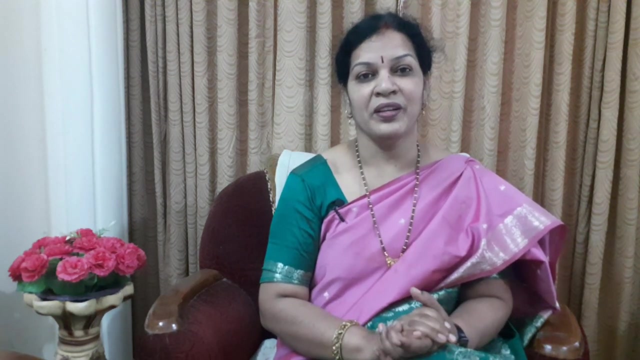 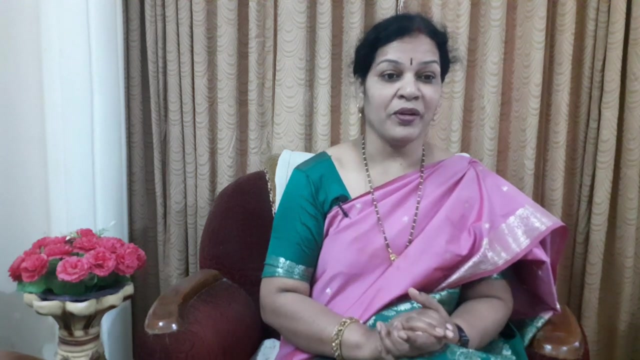 keep your ego rough and very hard nature and all these things. keep it aside. always be cool and give them a confidence that whatever you are going to teach the students are going to understand. that kind of assurance to give it to them, then automatically students will start loving your lectures. and always pleasing face is important. 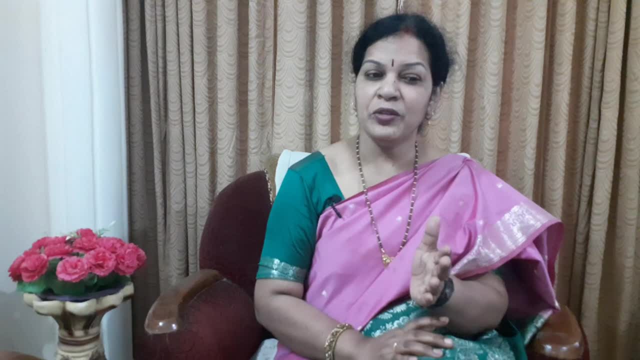 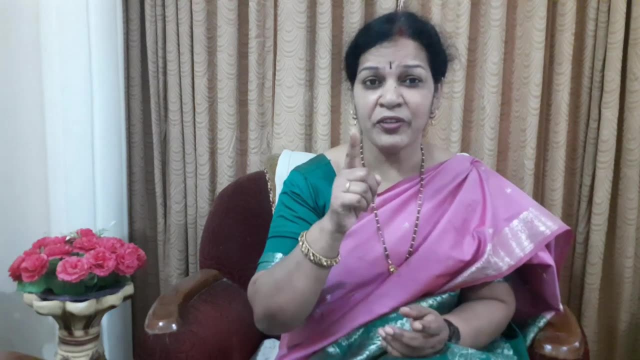 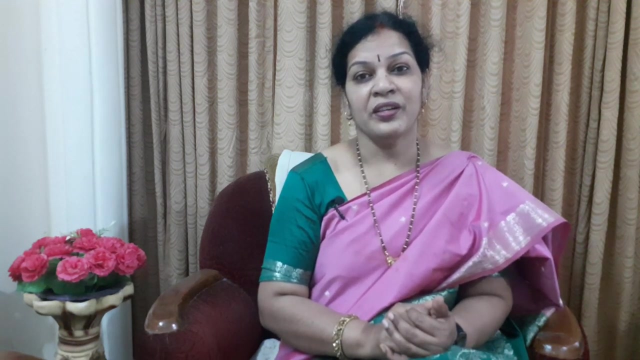 in that way you keep it and, at the same time, your attitude along with attitude, appearance- appearance also matters a lot, especially young teachers are telling you, whatever may be your age, just a completed post graduation and your age is maybe 22, 23, whatever may be your age, you. 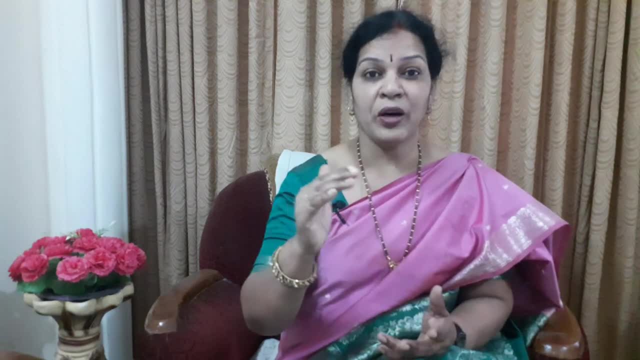 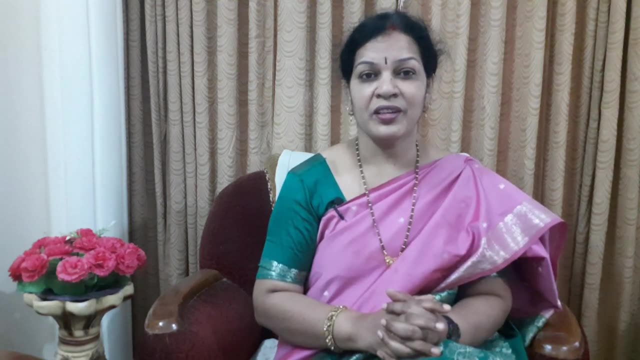 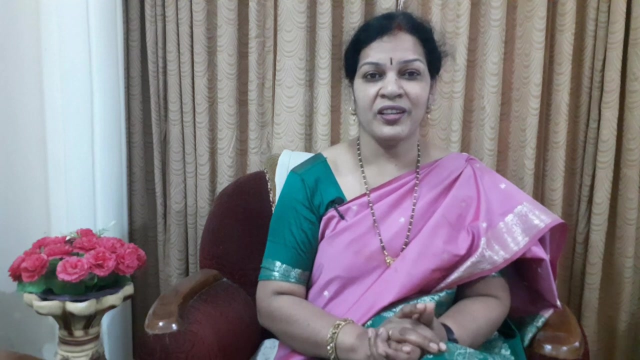 should look dignified, decorum you have to maintain, so that professional appearance is important. I have seen in some of the colleges, the faculty and faculty- Lady faculty- they used to come with loose hair and clothes, also not professional. so what you are going to teach to the students if your 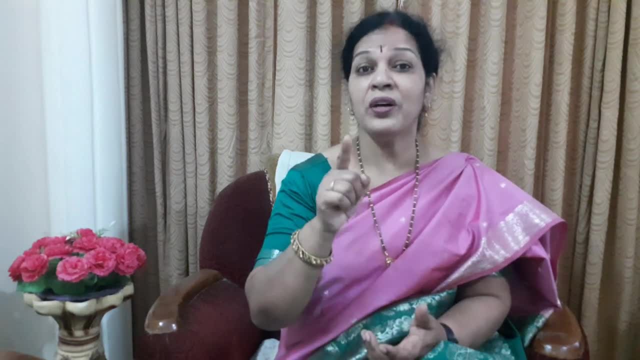 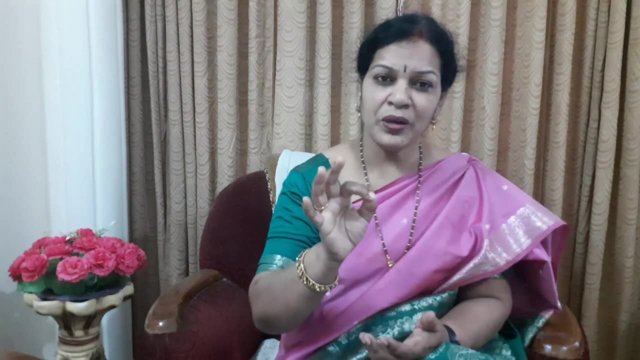 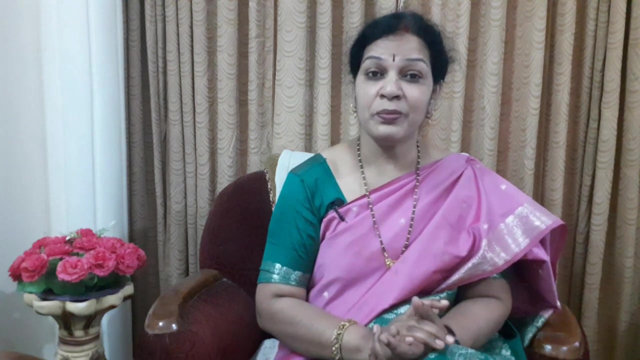 appearance is like that. so should the students focus on you or on your subject? I am asking you question, so that is where, please remember, you have to attract the students only with your knowledge and subject, not with anything. maintain the decorum dignified, so that kind of appearance, that's very much. 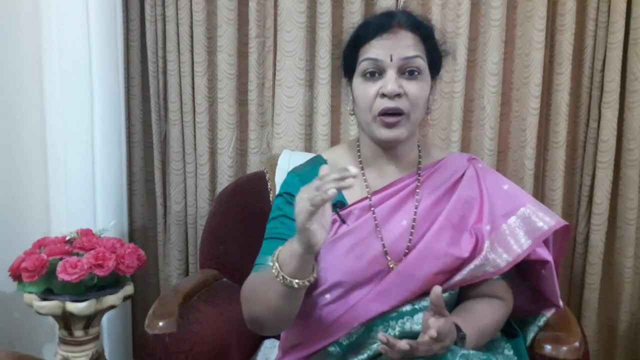 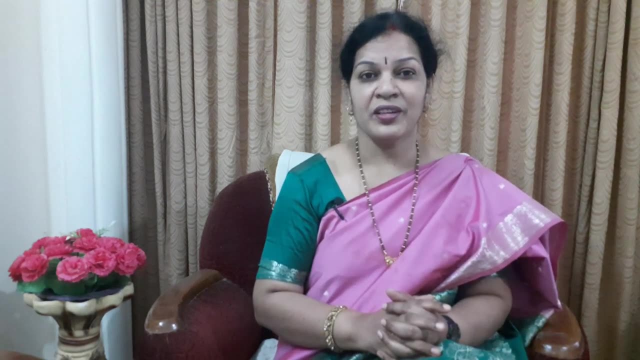 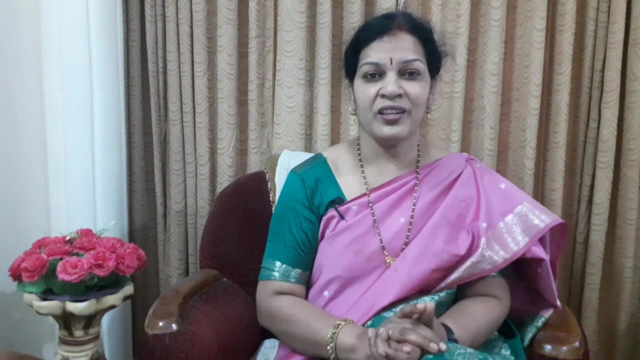 should look dignified, decorum you have to maintain, so that professional appearance is important. I have seen in some of the colleges, the faculty, young faculty, lady faculty- they used to come with loose hair and clothes, also not professional. so what you are going to teach to the students if your 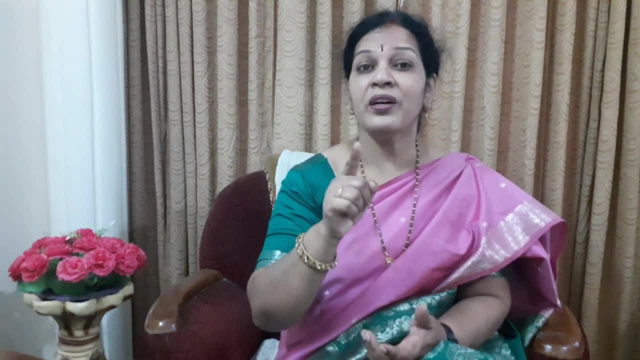 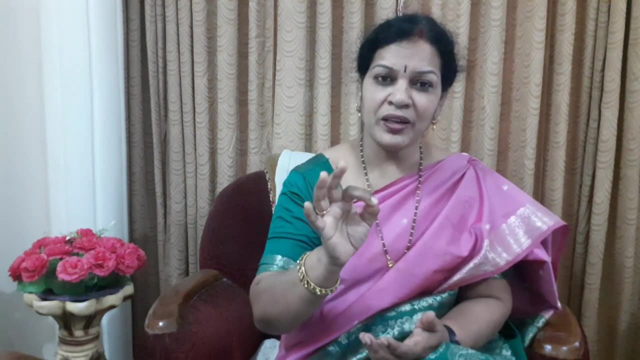 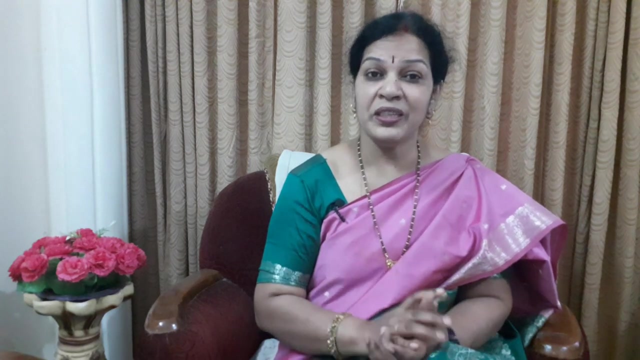 appearance is like that. so should the students focus on you or on your subject? I am asking you question. so that is why please remember you have to attract the students only with your knowledge and subject, not with anything. so always maintain the decorum dignified, so that kind of appearance that's very much important, decent. 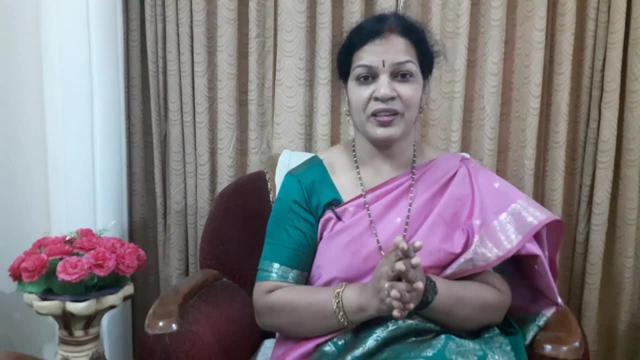 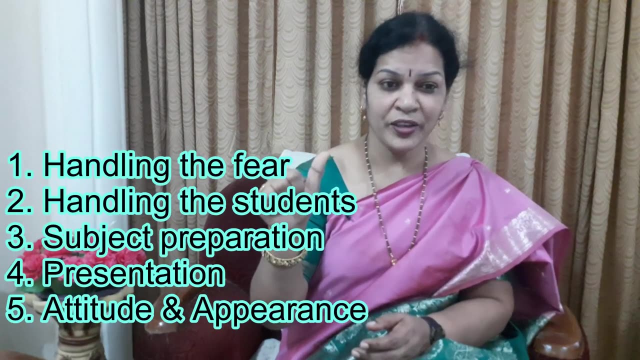 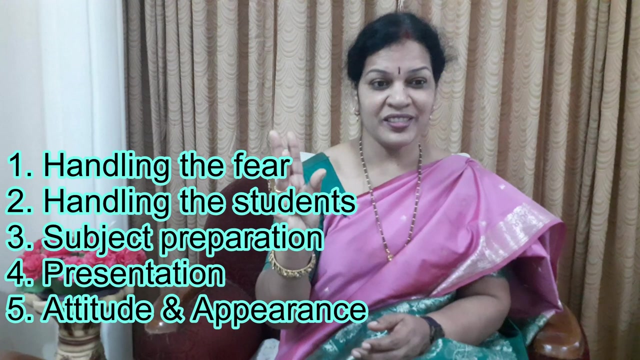 clothes, decent colors, so that you have to wear. so these are the simple five things I wanted to tell you. let me give you a recap. recap: first thing is that handle the fear and handling the students and subject preparation is important: presentation and communication skills and attitude and appearance. 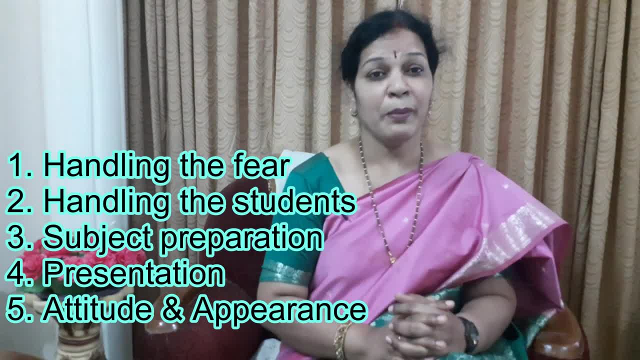 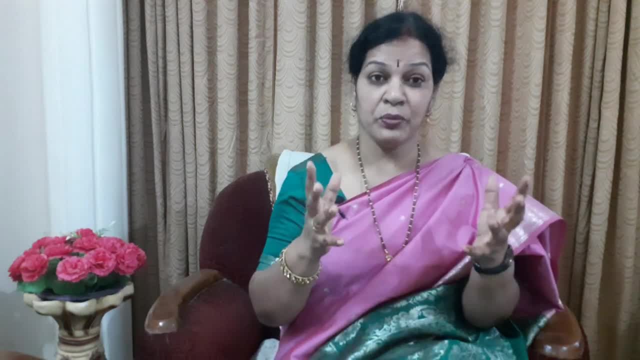 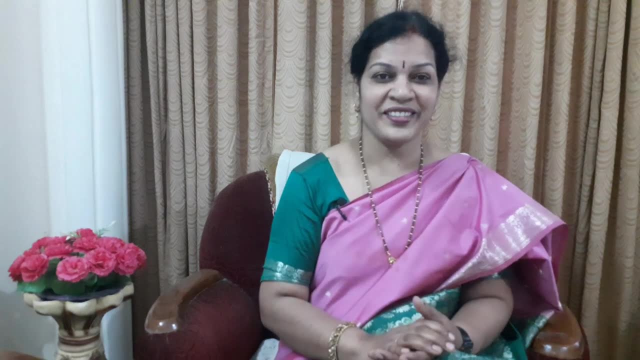 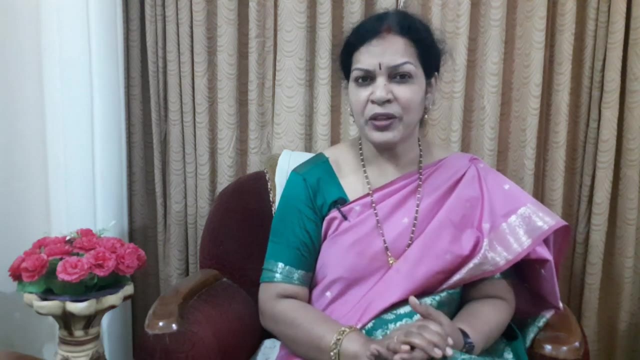 sometimes you know that the class look dull, but never keep the class dull. always the class should be vibrant and the class should be vibrant. there are some strategies to keep your class vibrant. I'll tell you some of my strategies. what I used to teach to the MBA students: if the class was 50 minutes out of 50 minutes, I used to. 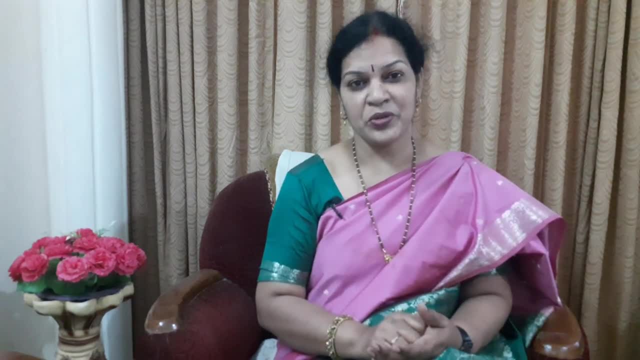 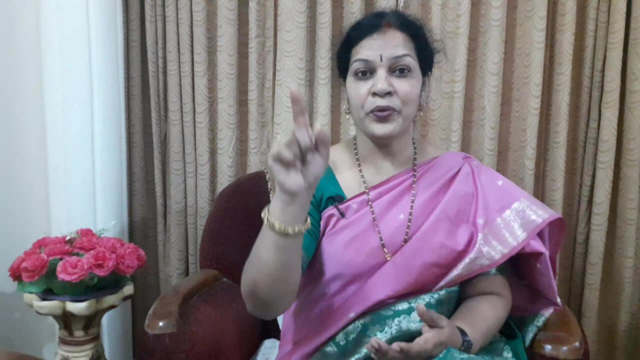 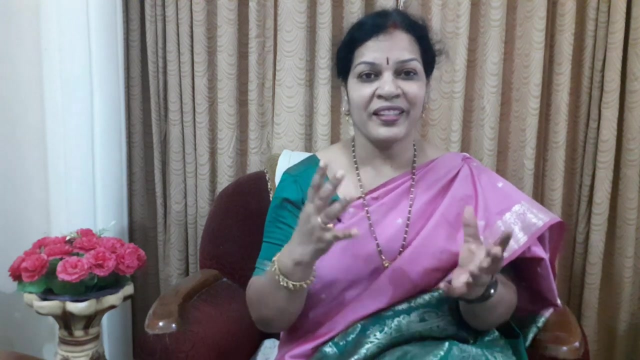 teach only 30 minutes only. but before 30 minutes I used to announce in the classroom that after 30 minutes of my talk, the rest of the 20 minutes any of you are going to explain it's my choice. I may ask anyone to explain the same topic. then entire class used to be very much alert maybe. 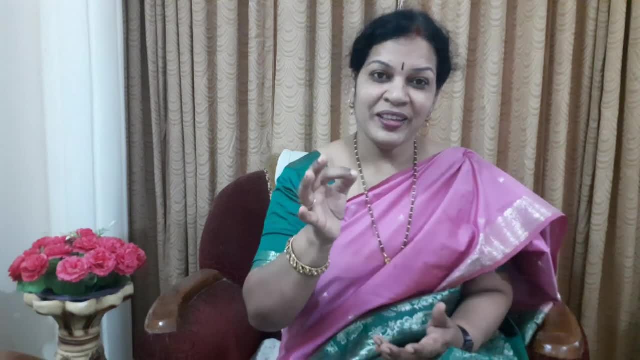 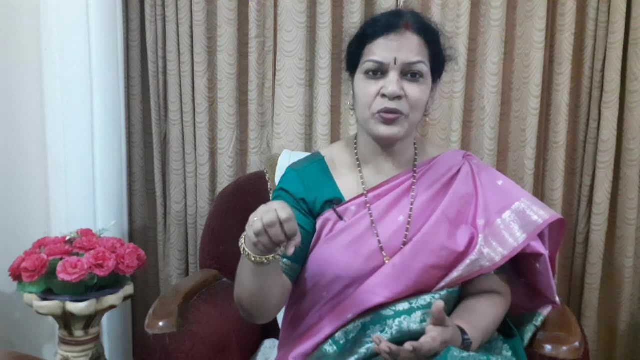 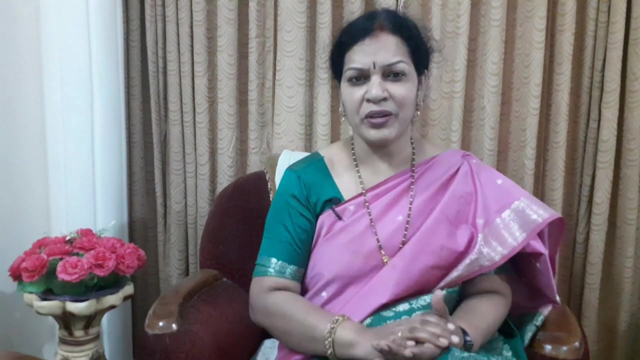 my turn, I have to explain. so in that way, teach the class and keep them a vibrant atmosphere. and when you call the students to explain the topic, so don't be so harsh. be friendly and encourage them. why are you scaring about the other students? they are just your. 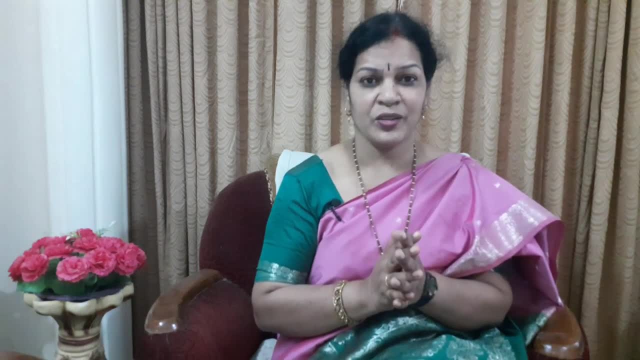 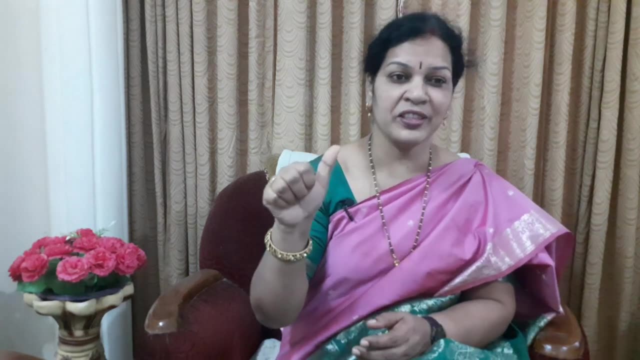 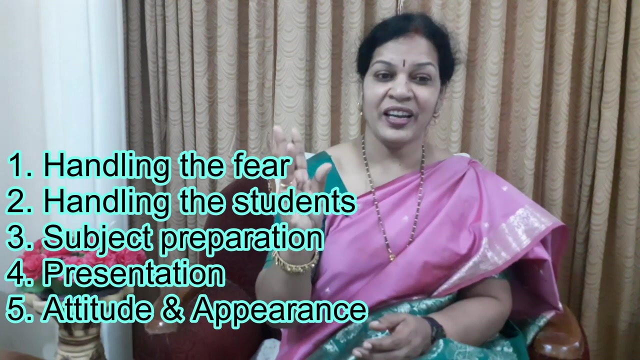 important: decent clothes, decent colors, so that you have to wear. so these are the simple five things I wanted to tell you. let me give you a recap. recap: first thing is that handle the fear and handling the students and subject preparation is important: presentation and communication skills and attitude. 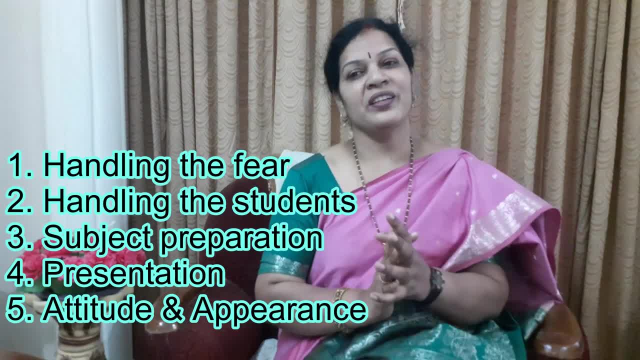 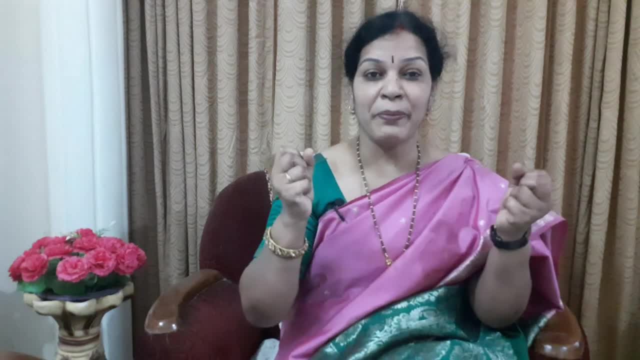 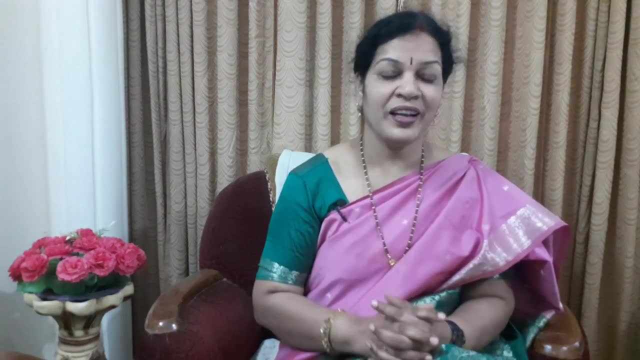 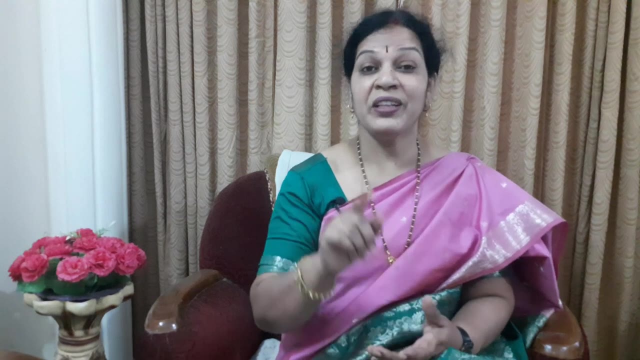 and appearance. sometimes you know that the class will look dull. but never keep the class dull. always the class should be vibrant and the class should be vibrant. there are some strategies to keep your class vibrant. I'll tell you some of my strategies. what I used to teach to the MBA students: if the class 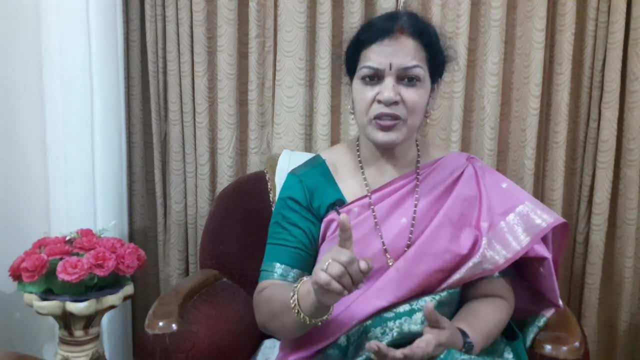 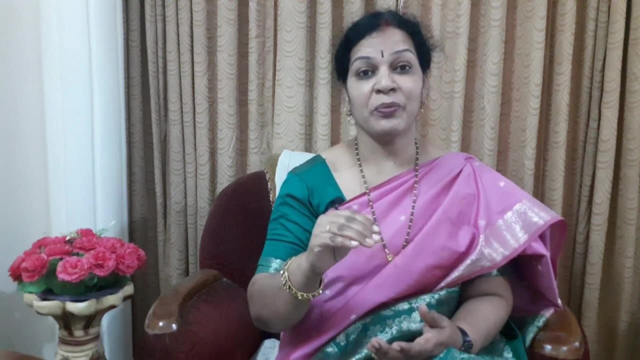 was 50 minutes out of 50 minutes. I used to teach only 30 minutes only. but before 30 minutes I used to announce in the classroom that after 30 minutes of my talk, the rest of the 20 minutes any of you are going to explain it's my. 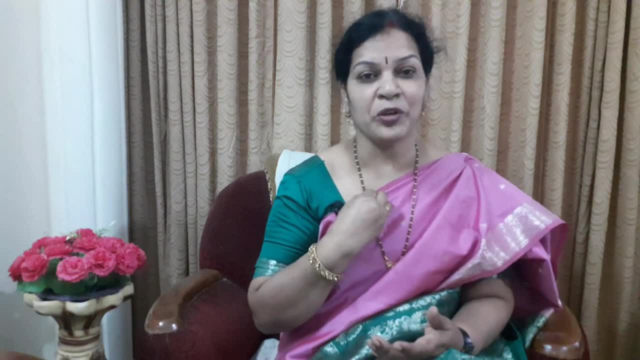 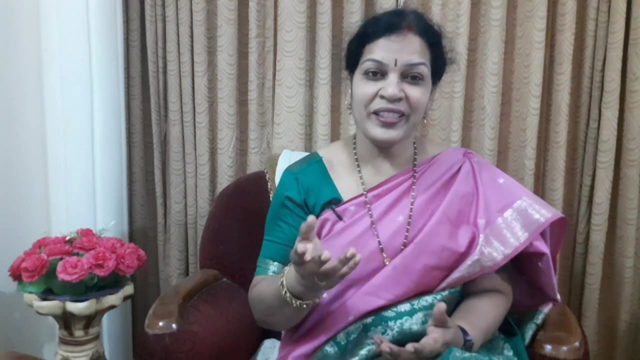 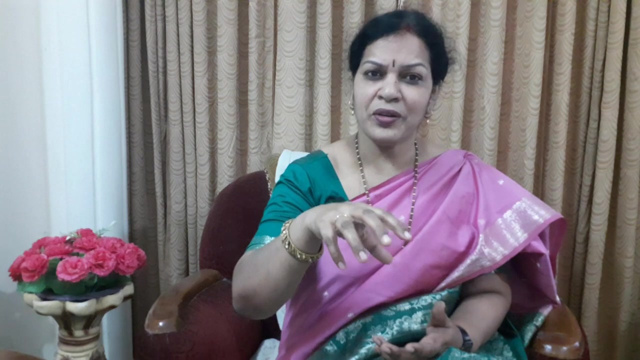 choice, I may ask anyone to explain the same topic. then entire class used to be very much alert. maybe my turn I have to explain. so in that way, teach the class and keep them a vibrant atmosphere and when you call the to explain the topic, so don't be so harsh. be friendly and encourage them. why? 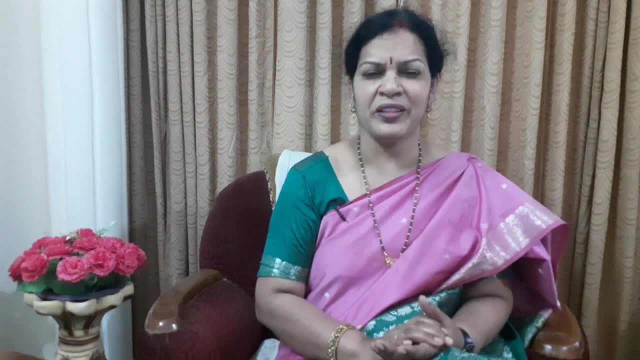 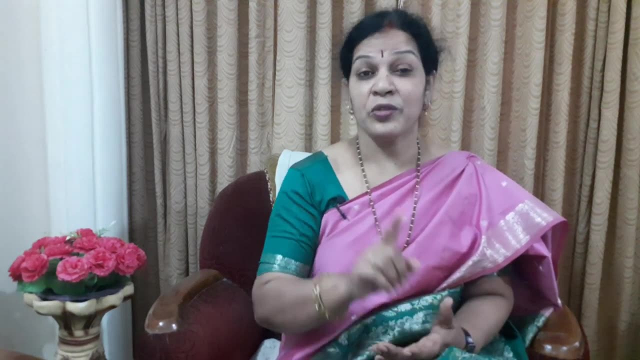 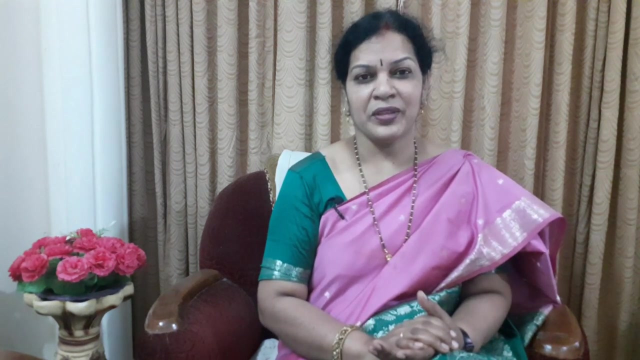 are you scaring about the other students? they are just your friends. only, they don't in fact anything. you know everything. you come and start it in that way. you have to encourage the student. so this was one of my strategy, and another strategy I'll tell you. sometimes, after lunchtime, the class will be dull. 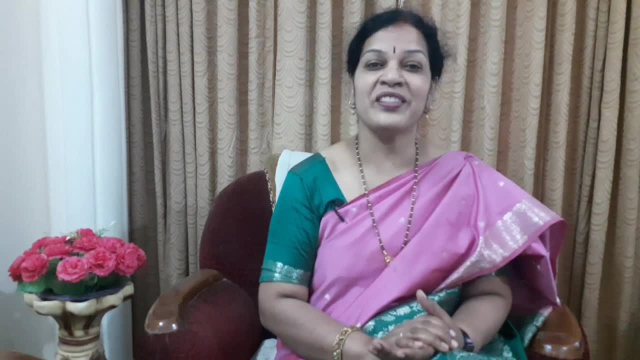 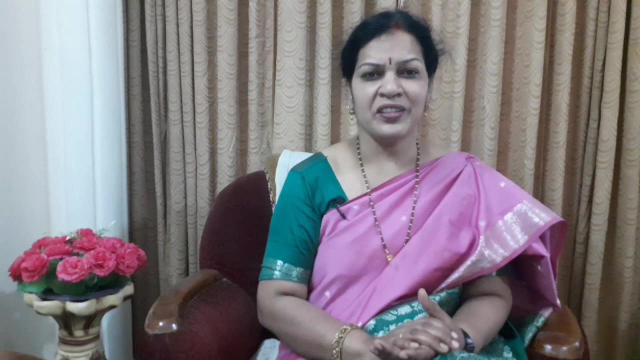 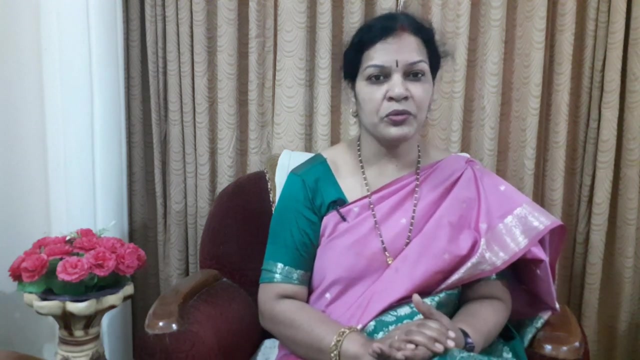 students, not only students. faculty also sometimes feels drowsy. so at that period what you have to do is start the class with any interesting question, general knowledge, puzzle or anything. start with a vibrant atmosphere. if you are dull, the students will sleep in the classroom by opening the eyes. that is why always, 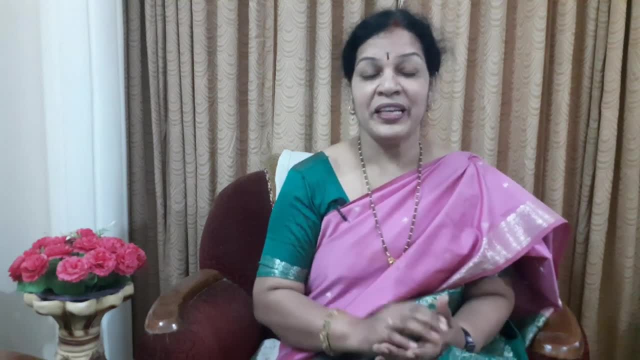 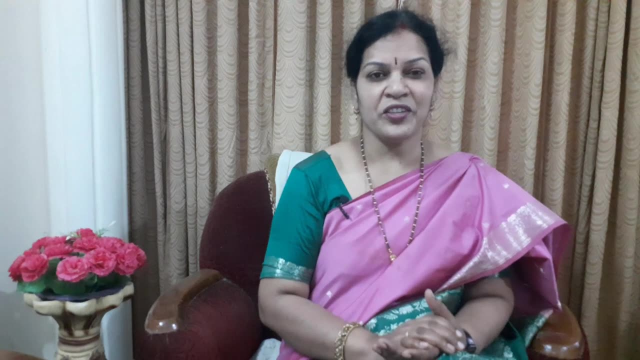 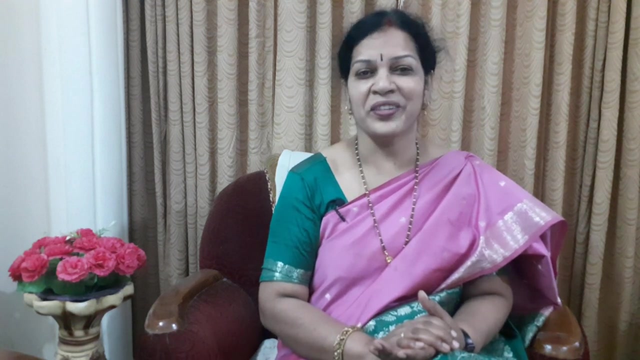 friends. only they don't in fact anything. you know everything. you come and start it in that way. you have to encourage the student. so this was one of my strategy. and another strategy I'll tell you: sometimes, after lunch time, the class will be dull. students, not only students, faculty also. 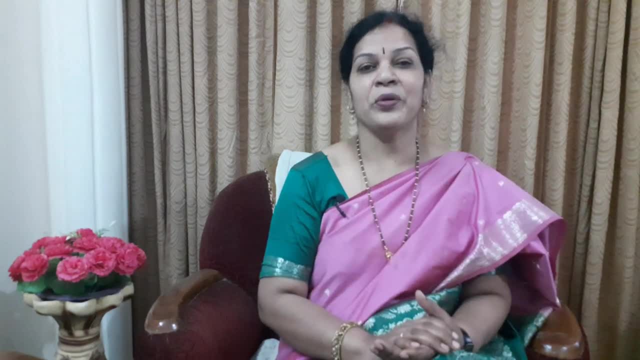 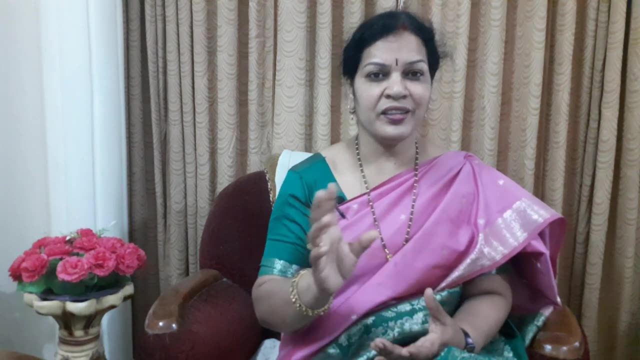 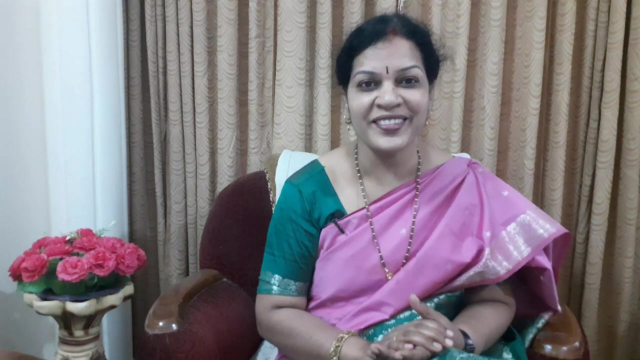 sometimes feels drowsy. so at that period what you have to do is start the class with any interesting question, general knowledge, puzzle or anything. start with a vibrant atmosphere. if you are dull, the students will sleep in the classroom by opening the eyes. that is why always start. 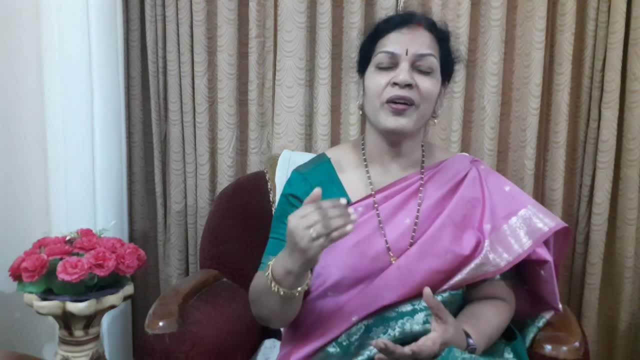 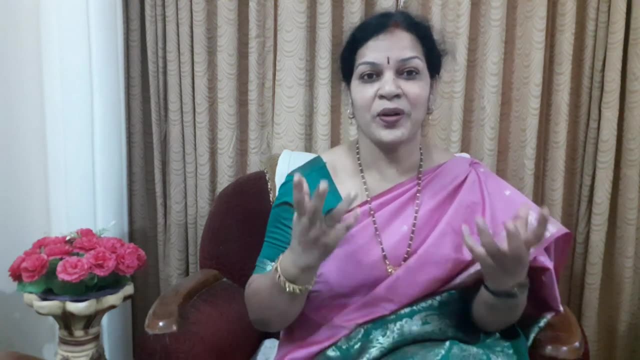 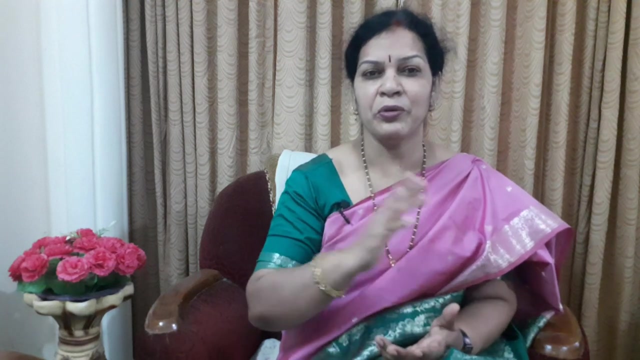 vibrantly and keep on asking small questions, minor questions you can ask the students so that they'll respond. if they don't respond, make them to alert and ask them: why are you not giving the answers? what's wrong which you come and be active like? you have to use good language and motivate. 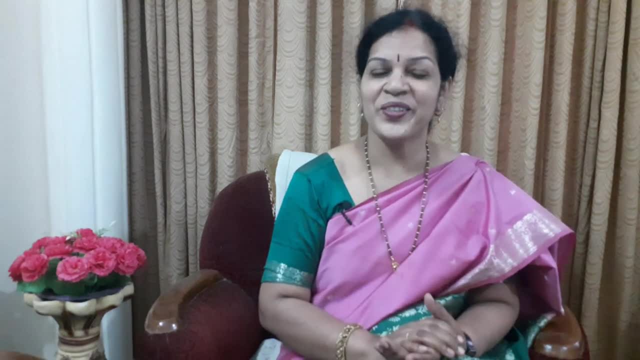 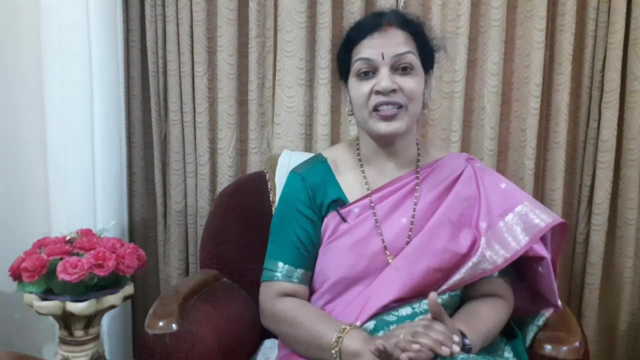 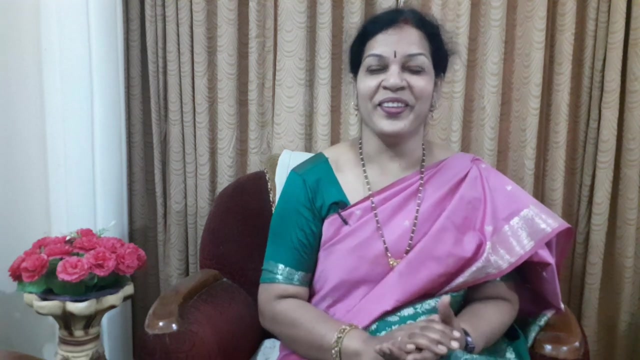 the student. this I used to do sometimes. you know what I used to do. sometimes I used to ask a question. what did I say? just repeat it. I don't want any answer. whatever I said, repeat just now. what was my last sentence, repeat it. then students used to feel: oh, we have to be alert. so, in that way, be friendly and 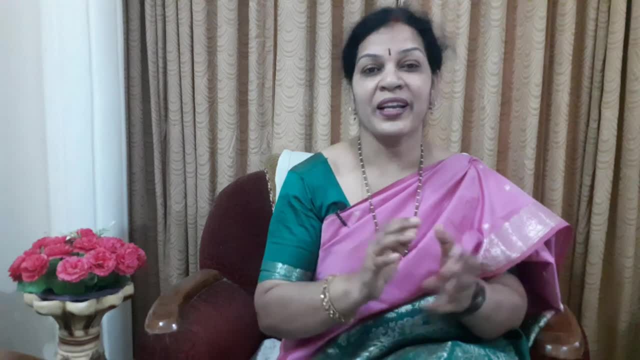 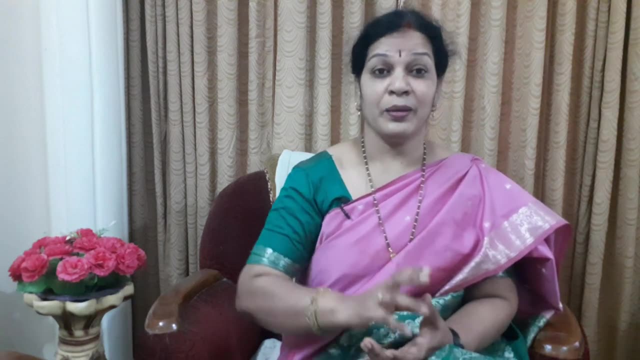 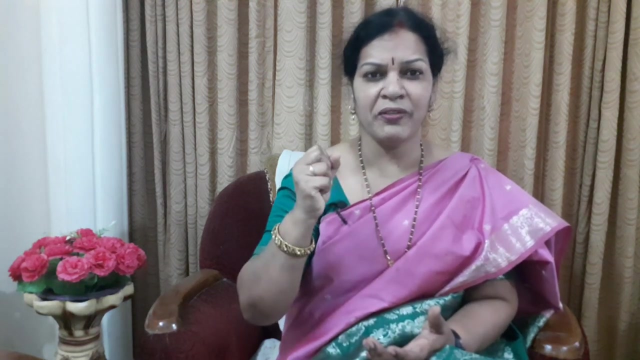 keep the class vibrant and also during the class. you can crack some natural jokes, also by taking examples and by using a funny language. but it should not deviate the mind of the students. to attract the students, to keep the class vibrant. for that purpose you can crack some kind of jokes related to the 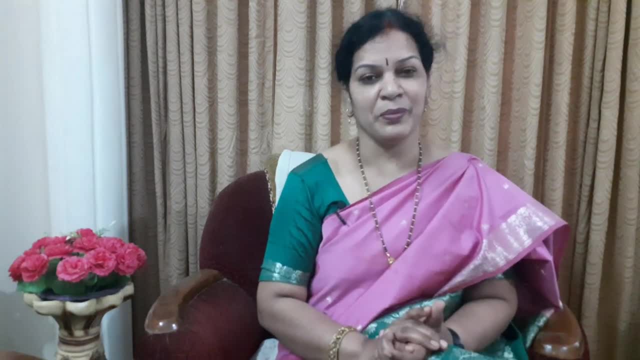 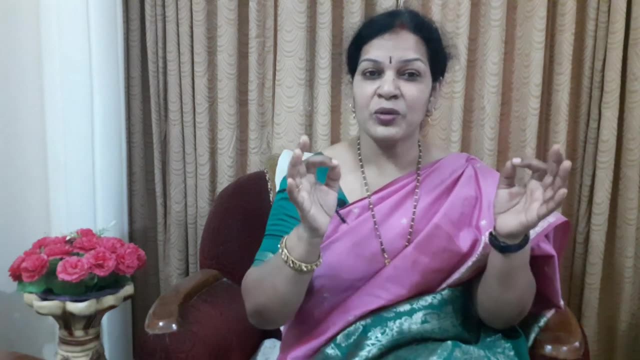 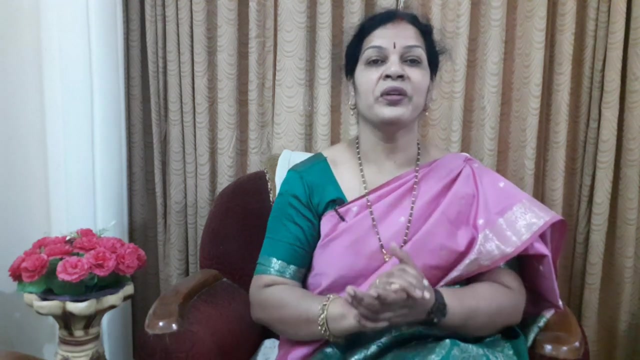 subject. a little bit out of the subject also doesn't matter and related to the students also you can take, so in that way you can keep the entire class vibrant slowly. if you are a new faculty it will take some time- hardly one year or two year after that you get a. 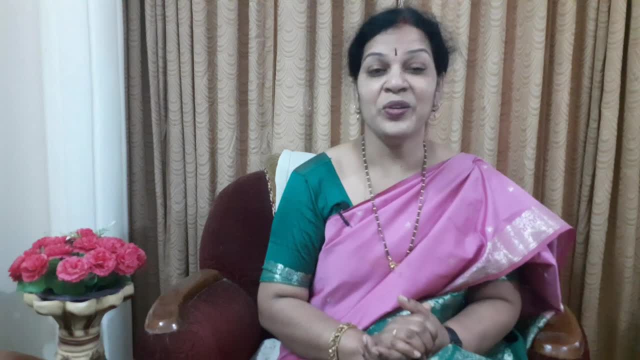 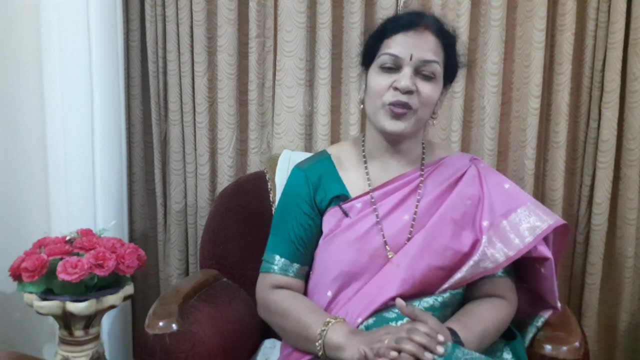 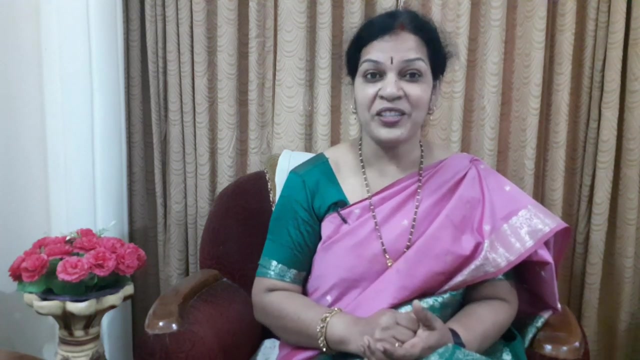 lot of command. you will tell me. you are going to say, ma'am, I am been handling class like this and this is my strategy, this is my style. so students will love you a lot if you have a good strategy of teaching, with some subject command and good attitude, good appearance. these are the 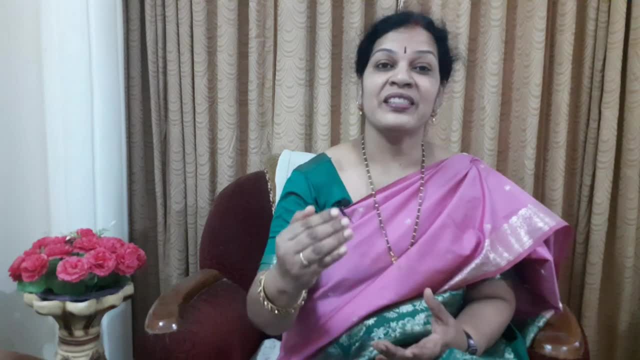 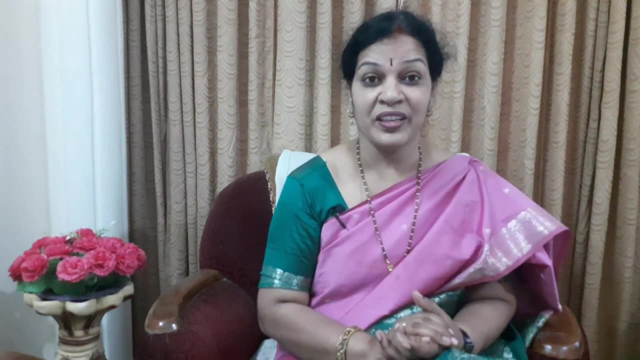 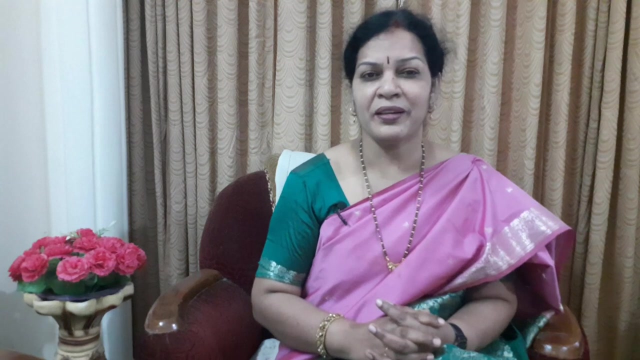 start vibrantly and keep on asking small questions, minor questions you can ask the students so that they'll respond. if they don't respond, make them to alert and ask them: why are you not giving the answers? what's wrong with you? come and be active, like you have to use good language and motivate the student. 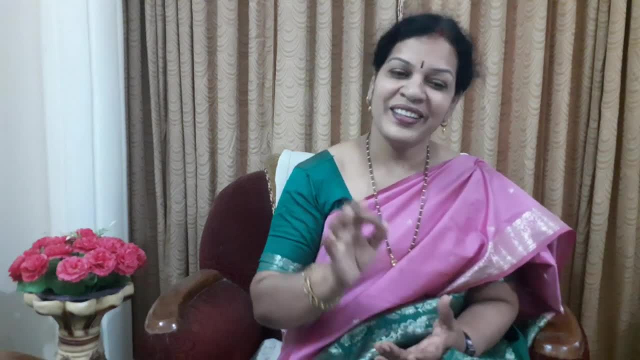 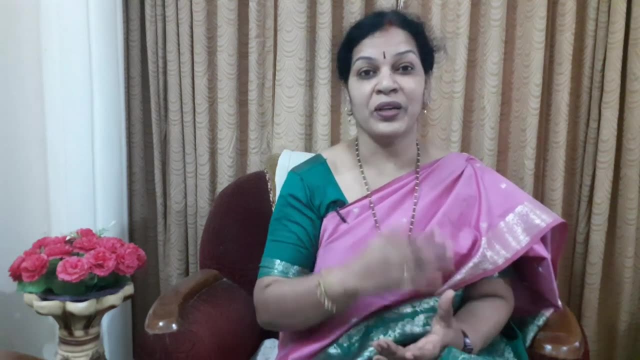 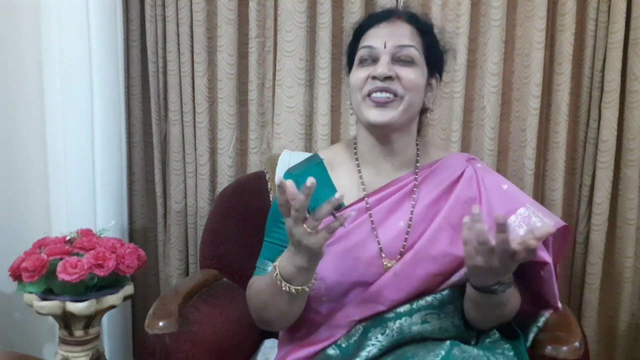 this I used to do sometimes. you know what I used to do. sometimes I used to ask a question: what did I say? just repeat it. I don't want any answer. whatever I said, repeat just now. what was my last sentence? repeat now it. then students used to feel: oh, we have to be alert. so in that way, be friendly. 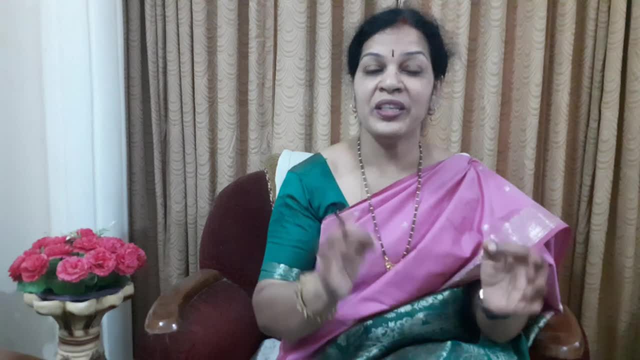 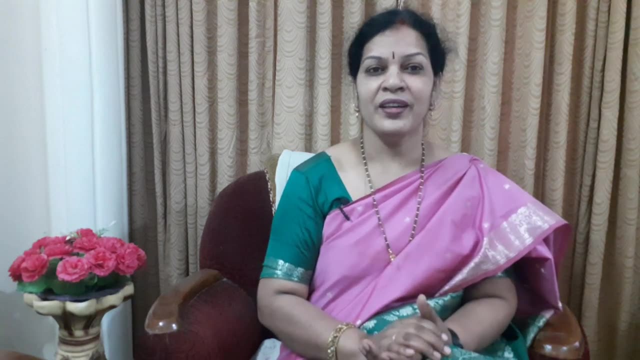 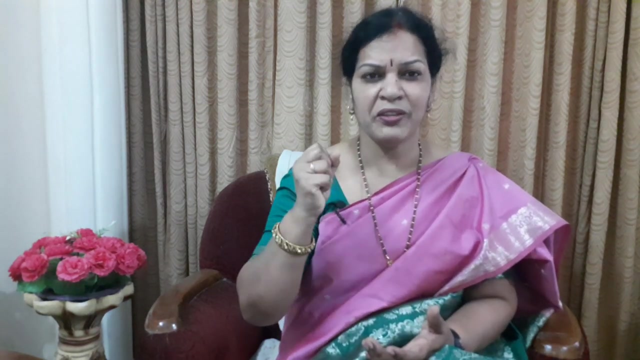 and keep the class vibrant and also during the class you can crack some natural jokes, also by taking examples and by using a funny language. but it should not deviate the mind of the students. to attract the students, to keep the class vibrant. for that purpose you can crack some kind of jokes related to. 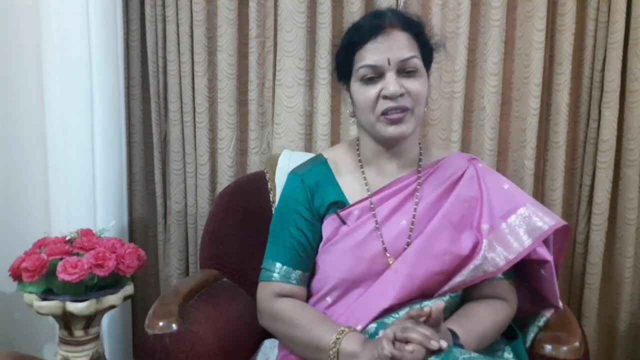 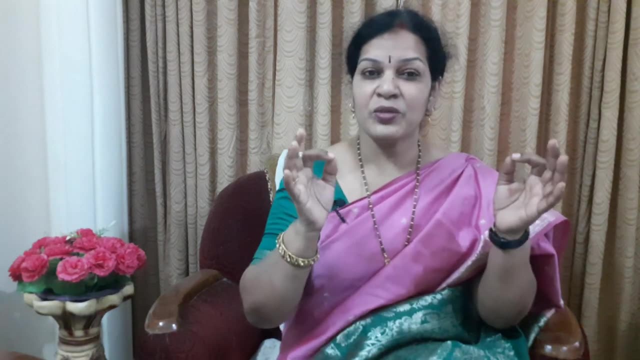 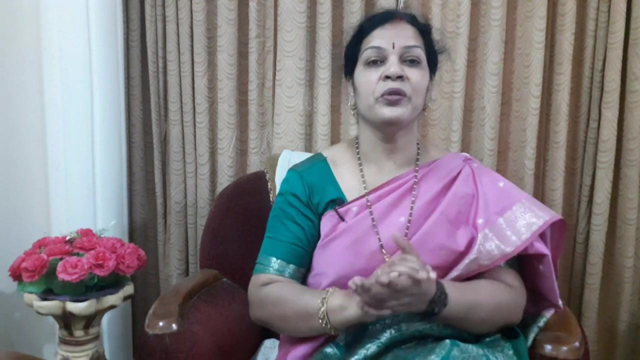 the subject. a little bit out of the subject also doesn't matter and related to the students also you can take. so in that way you can keep the entire class vibrant slowly. if you are a new faculty it will take some time- hardly one year or two year. after that you get a lot of command. you will tell me you are going. 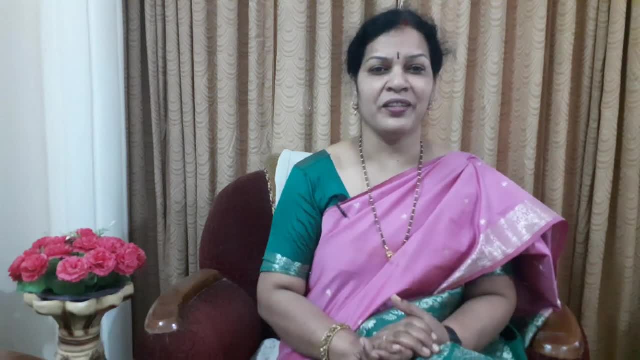 to say: ma'am, I'll, I'm been handling things very well and I'm going to do something very well. and I'm going to do something very well and I'm going to do something very well and I'm going to class like this and this is my strategy, this is my style, so students will love. 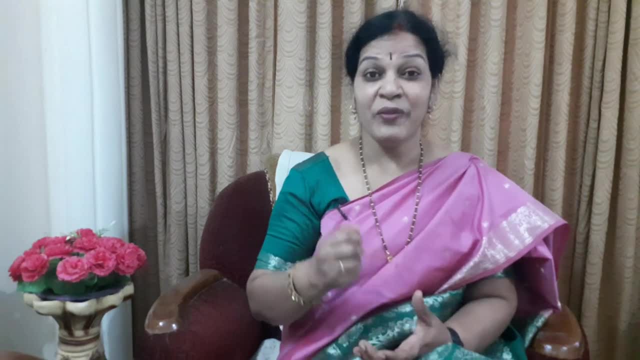 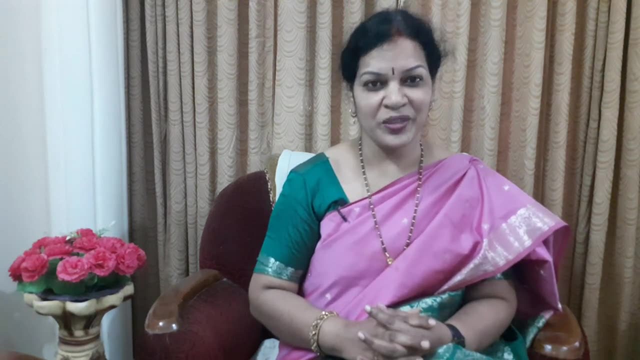 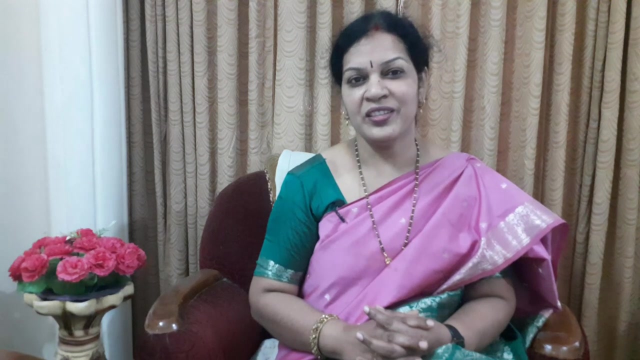 you a lot if you have a good strategy of teaching with sort of subject command and good attitude, good appearance. these are the simple things. hope my dear angst or young faculty members and teachers and lectures, please follow this and never hesitate. you are going to change the generations. we have that.